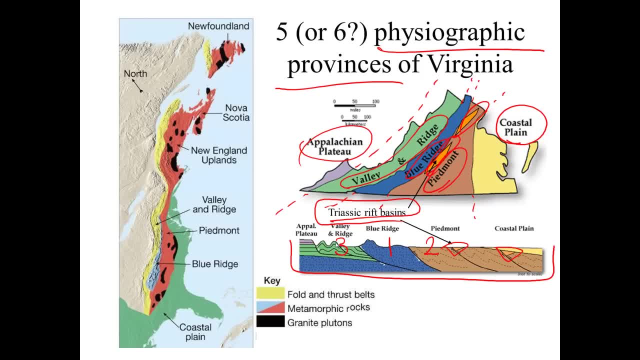 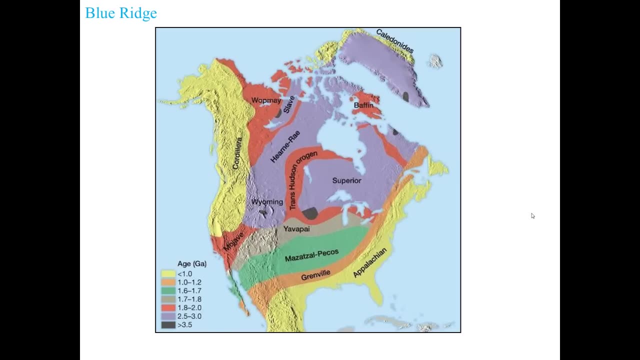 Chapter 3 kind of tells the same story as Chapter 2, except from a very different perspective. And then we go into Chapter 4 with the Appalachian Plateau, Chapter 5 with the rift basins, and then Chapter 6, the Coastal Plain, tells the end of the story. 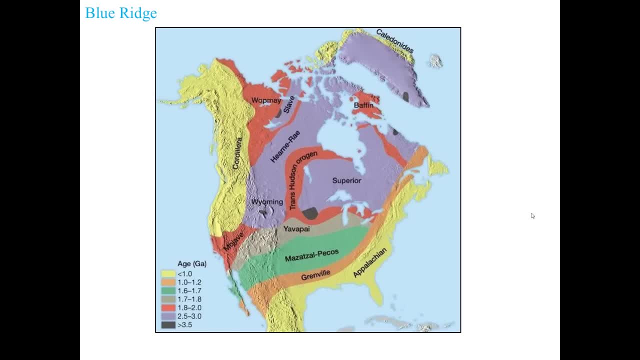 Zooming out even further, you can see that Virginia's geological history is part and parcel of the geological history of the entire continent of North America. This is a map of North America that's color-coded to show the age of the crust in different regions of the continent. 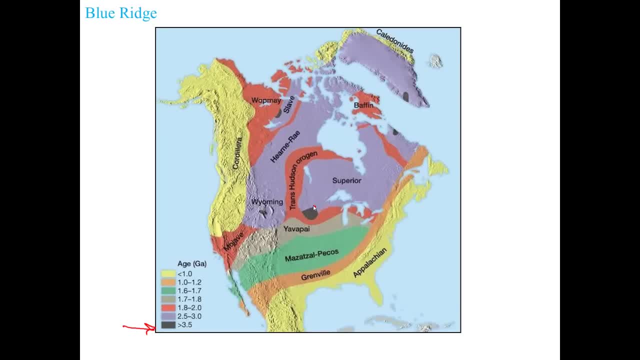 The oldest crust is a sort of gray color and you can see there's a blob of it here in Minnesota, a blob in Wyoming, a blob up in the Northwest Territories and another blob that's been split in half, part in Greenland, part in Labrador. 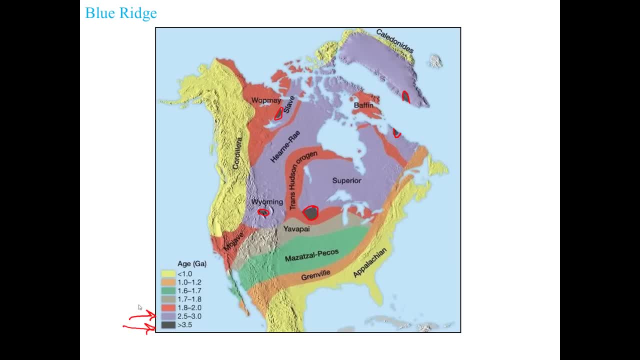 So those old blobs are surrounded by progressively younger and younger crust And you can see that basically these are sort of proto-continents that glommed on to one another so they smashed into one another and then they stuck. So the Trans-Hudson origin there in red that is basically an old mountain belt. 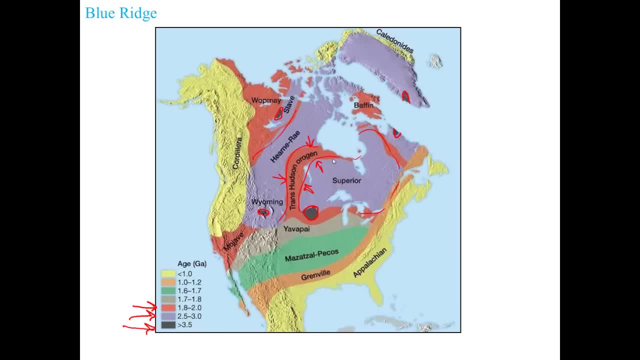 where the Hern-Rey Province collided with the Superior Province. Then additional accretions of new material tacked on to the southeast- You can see the Yavapai, the Mazatzal, Pecos and the Grenville, And then the very youngest rocks, basically, are tacked on the outboard side of that. 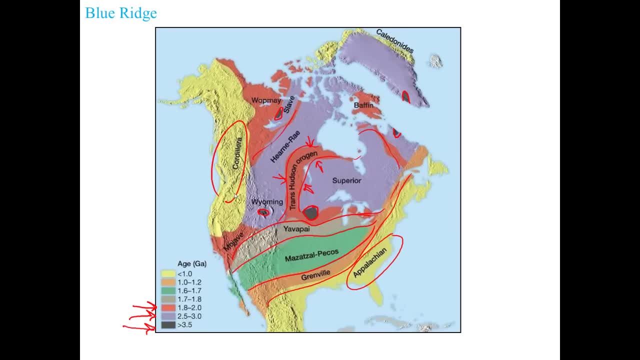 So this overall pattern is sort of like building a snowball: You start by packing snow in and then you add more and more snow on the outside to make your snowball bigger. In the same way, here you start with small pieces of old crust. 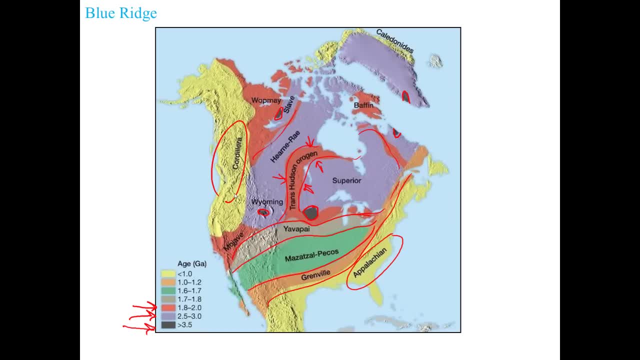 and then you tack on progressively more and more crust, making the final blob of crust- the continent- even bigger. So Virginia's geological story basically involves snow. It's two of these: the Grenville piece and then the Appalachian piece. So let's take a look at those. 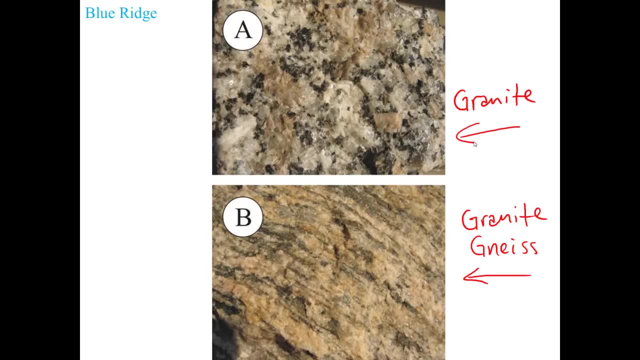 The oldest rocks in Virginia are granites and granite gneisses of the Blue Ridge Basement Complex And in general. our granite gneisses are around 1.1 billion years old, or giga-annum, And the granites are around 1.0 billion years old or giga-annum. 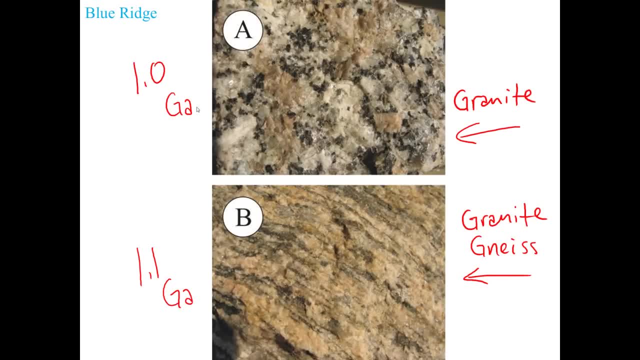 So that GA abbreviation means billion years ago, The granites formed during an ancient episode of mountain building called the Grenville Orogeny. The Grenville Orogeny is named for a town in Quebec up in Canada, but its rocks are also found all the way down into as far as Texas and they come through Virginia as well. 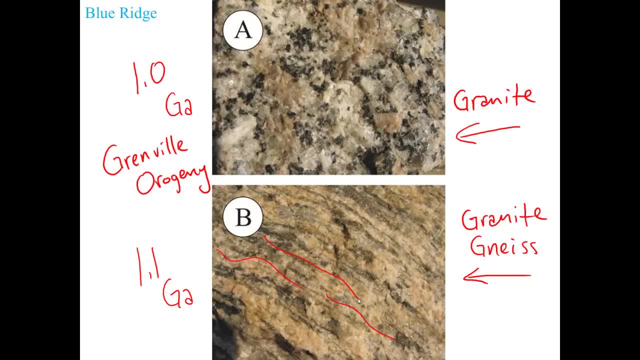 The granites that formed early in that orogeny then got squeezed and they developed a metamorphic foliation gneissic banding that squishes and squeezes through those granites. The granites that came in later in the orogeny did not get squeezed as much. 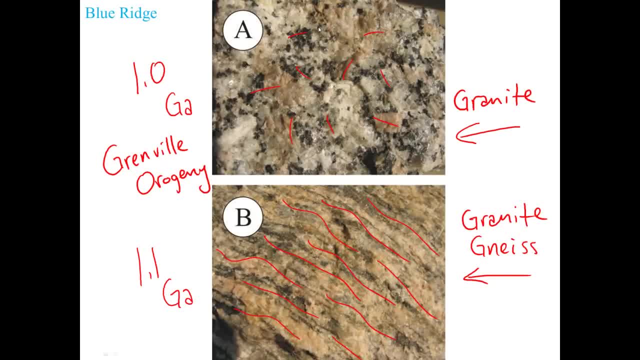 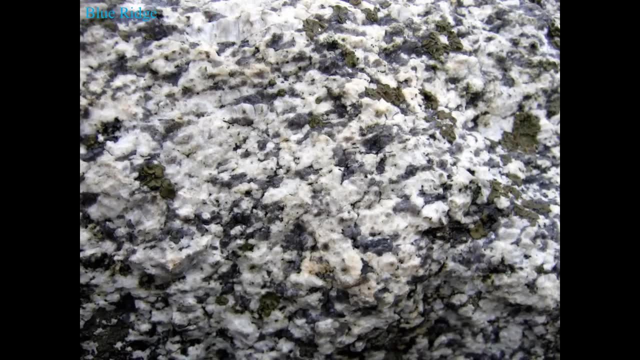 and so their crystals are sort of randomly oriented. An example of one of the granites is the Old Rag granite. This is a close-up look at the Old Rag granite. From one side of this picture to the other that's probably about 12 inches or so, about a foot wide. 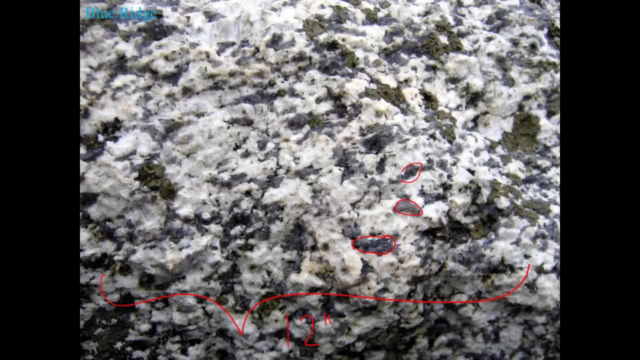 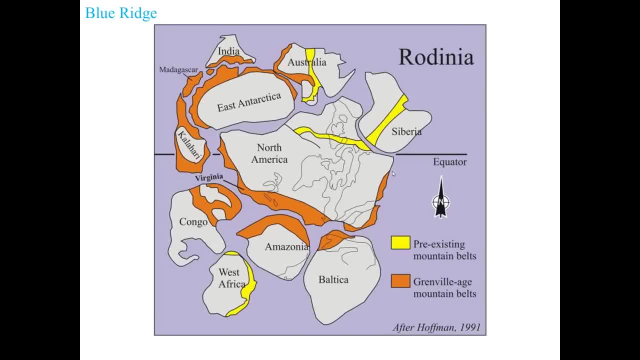 And you can see distinctive blue quartz crystals here. Those are typical of the Blue Ridge Basement Complex, as well as a lot of white feldspar. So the Grenville Orogeny is one of many orogenies that took place around the world at that time. 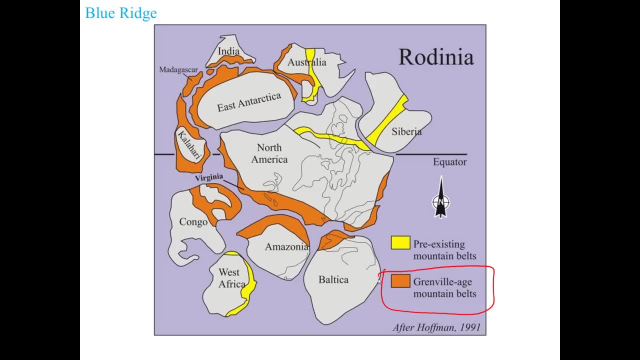 So on this map showing the situation around 800 million years ago, you've got these orange stripes showing where continents were smashing into one another. Virginia's location is right here and you can see that basically the strip of mountains would have run both off to what is today the northeast of here. 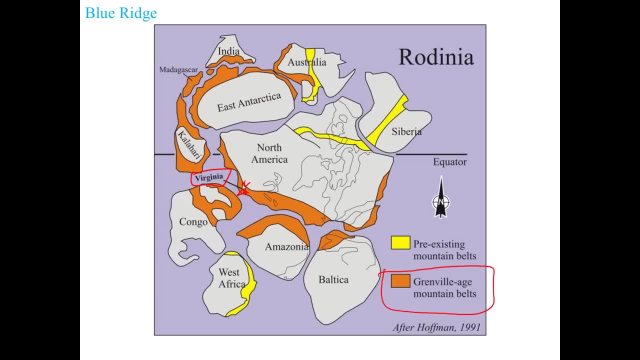 and off to the south. So off to the southwest, wrapping around Antarctica, India and Australia. Obviously, North America is no longer astride the equator today and it's no longer in this orientation. It has been rotated counterclockwise to get where we find it today. 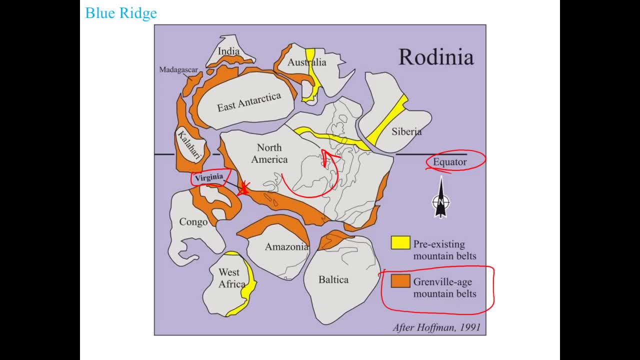 All of this mountain building that happened around a billion years ago assembled an early supercontinent known as Rodinia. So most people when they hear about supercontinents they think of Pangaea, but there was an earlier supercontinent, It was called Rodinia. 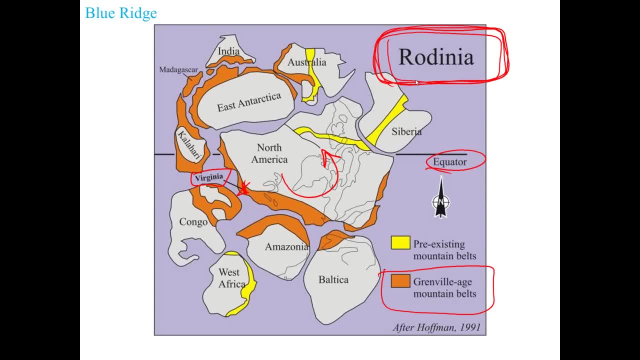 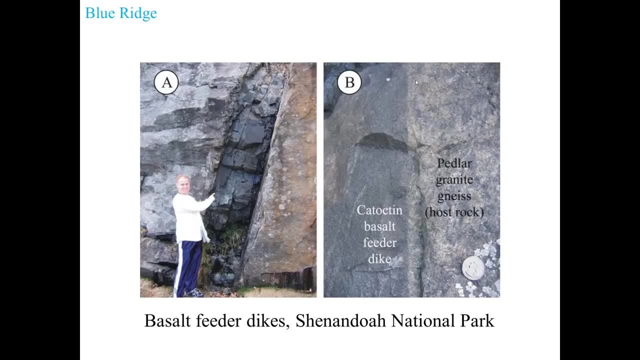 And it was built in the early 1800s And Virginia's oldest rocks record the assembly of Rodinia. Rodinia ultimately broke apart and that brought new rocks into the scene. Some of these rocks were mafic, igneous rocks. 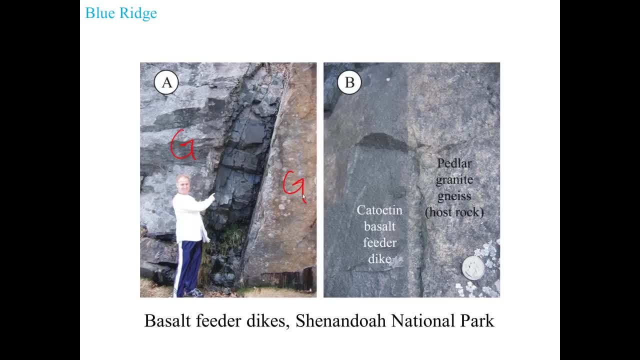 So what you have here are some of the granites that were associated with the Grenville Orogeny, And then they fractured open, and then, squirting through that fracture, came mafic lava, Lava that was poor in silica but rich in iron and magnesium. 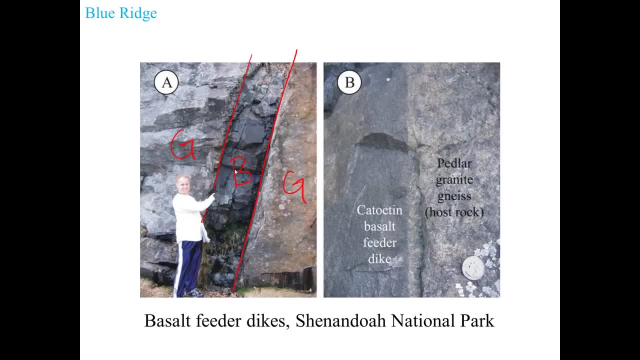 And so when it cooled, it became a basalt. If you look at the contact here, you can see. basically, there's a big difference between these basalts, which are around 570 million years old, and the granite gneisses, which are around 1.1 billion years old. 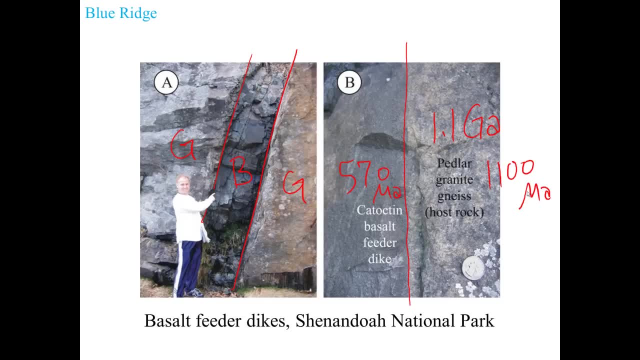 or 1,100 million years old, So there's a huge difference in age here. So at this time Virginia would have looked a lot like modern-day Ethiopia. So if you zoom in on Africa to Ethiopia, you'd see a scene that looks something like this: 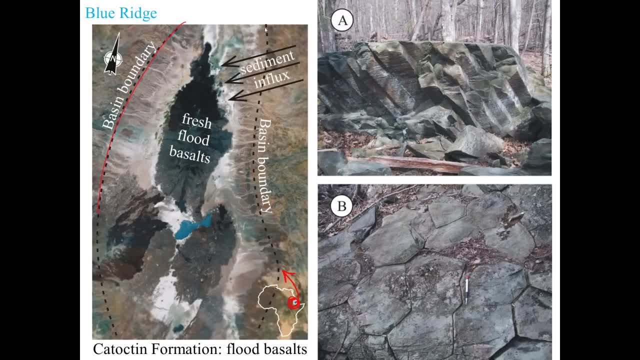 You've got a rift valley, And this rift valley is bounded by faults. Sediments pour off the surrounding highlands into the basin, the rift basin that's in between, And then there are these huge eruptions of mafic lava onto the surface. 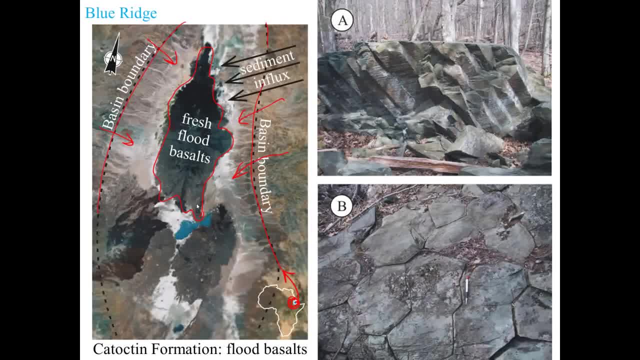 so-called flood basalts. When those flood basalts cool, they contract and you end up getting columnar jointing. We have columnar jointing in our flood basalts as well, So you can see this sort of hexagonal shape here. 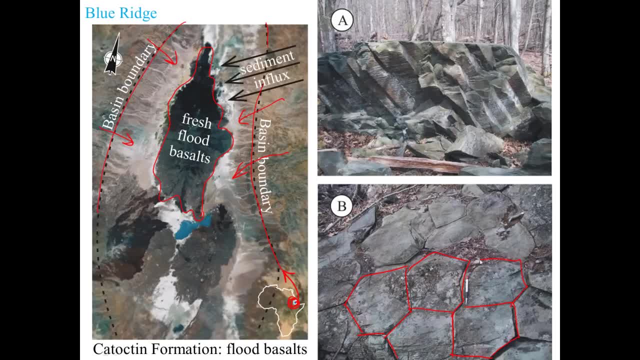 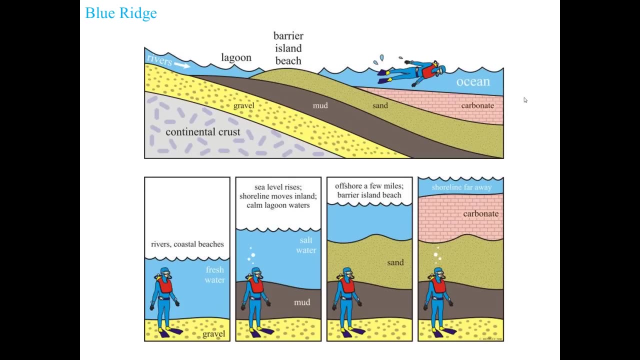 Between these blocks of what used to be basalt. This is exposed in Shenandoah National Park. If you look at these things from the side, you'll see that they have beautiful columnar shapes. Now, after Rodinia rifted apart, it opened up a new ocean basin. 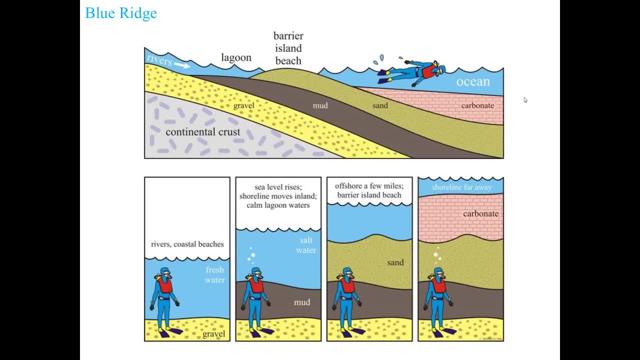 That ocean basin, called the Iapetus Ocean, existed between North America and the other continental fragments of Rodinia. So blocks of crust like the Congo Craton, the Amazonia Craton, ancestral Europe, ancestral Antarctica, that sort of thing. 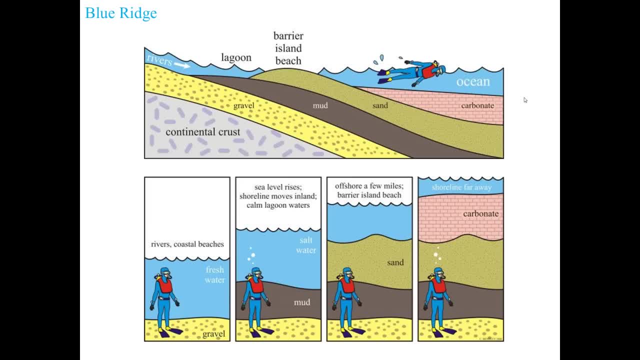 The edge of Virginia then cooled off because essentially Virginia, if you're looking at it from the side, had continental crust and then it's got this new and growing skirt of oceanic crust that's coming off of it out here in the Iapetus Ocean. 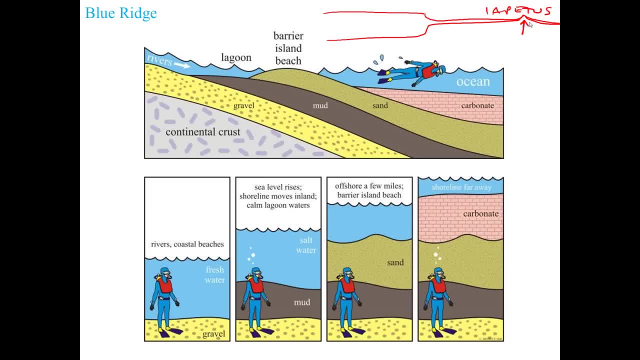 So there's an oceanic ridge there where new oceanic crust is being made, and Virginia is right here on the edge of the larger North American continent. So Virginia cools off, and as it cools off it condenses contracts. 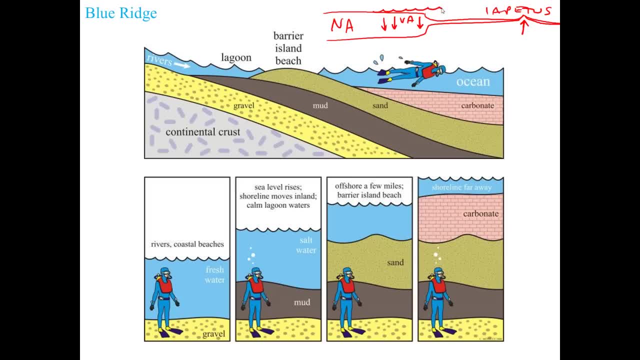 and that causes it to subside. That subsidence allows sea level to rise over the edge of the continental crust here in Virginia. As sea level rises, it brings with it a characteristic suite of sediments, and these sediments will be future sedimentary rocks. 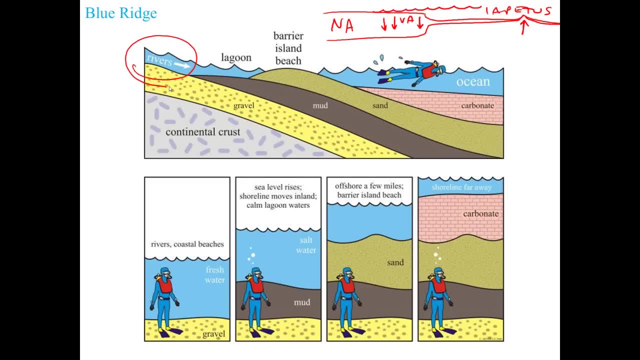 So, going from a near shore position, like where a river is flowing into the sea, to an increasingly offshore position, you would see first gravel and sand, then mud. that probably represents some sort of a lagoon kind of environment. Then there's some very pure. 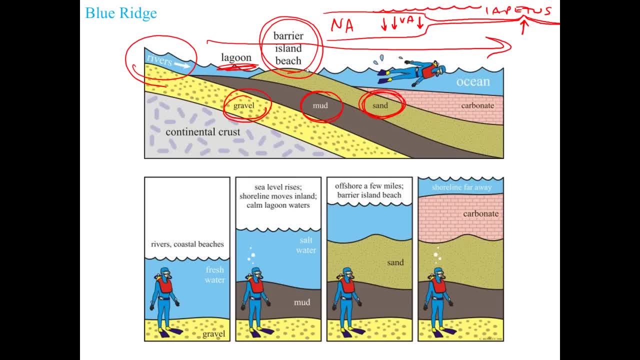 clean quartz sand that probably represents a barrier island complex, something kind of like the modern day outer banks of North Carolina. And then, if you get far enough away from the land, there's no more particles of sediment, and so you're only depositing chemical sedimentary rocks. 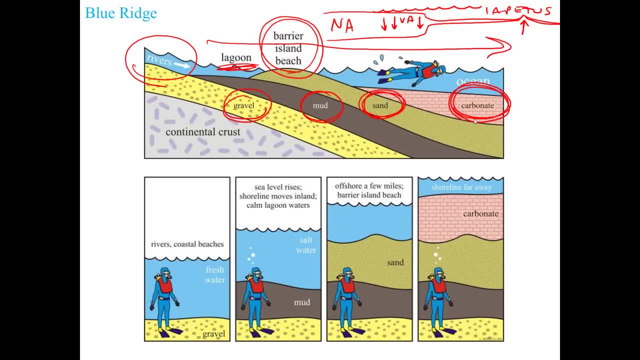 In other words, those sediments that crystallize directly from the seawater, such as limey mud and that's future limestone. Another way to think about this near shore to offshore sequence is to think of it from the perspective of a single place over time. 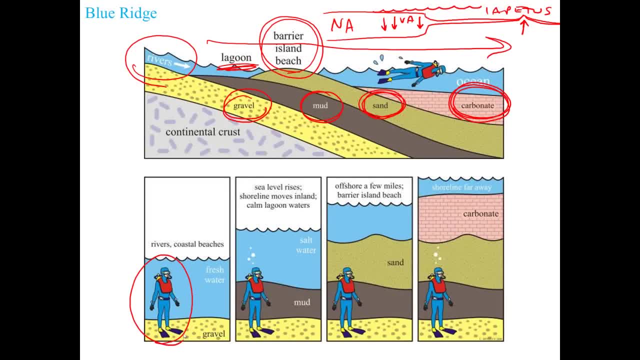 So imagine you went back in time. this is you here and you're wearing a scuba tank and you waded into one of these rivers that was draining the North American continent, flowing into the Iapetus Ocean. If you sat there and waded for long enough, 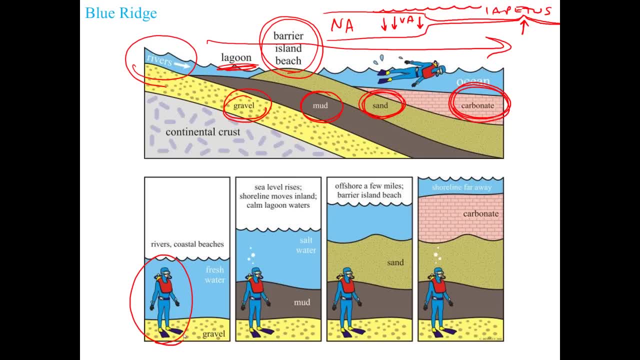 sea level rise at that location would bring all those different sediments to you. So you start off with the gravels and sands of the rivers and the beaches, Then a lagoon moves over your head and mud's deposited on your location. So that'd be like a Chesapeake Bay kind of scenario. 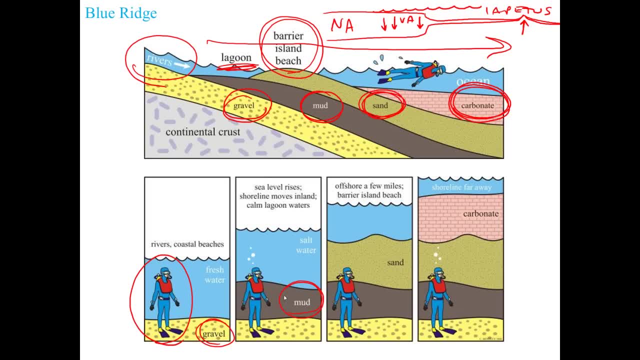 or Pamlico Sound, if you're familiar with North Carolina, Then those barrier islands move over your head and you get a bunch of sand deposited on top of the mud. And finally, when the shoreline is far, far away and sea level's at its highest, 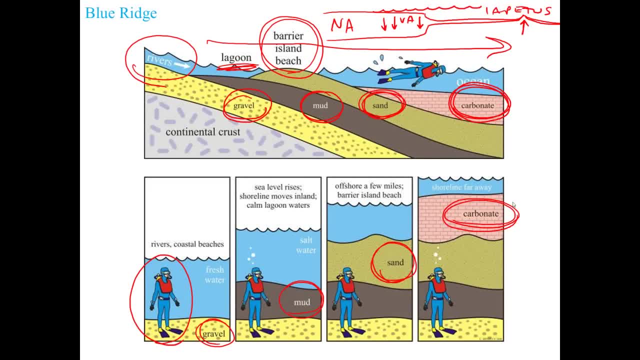 you end up getting the crystallization of the seawater and you end up getting limey mud deposited at that site, So that would be carbonate instead. Well, that whole sequence is exactly what we see in Virginia. So here's an example of some of the carbonates. 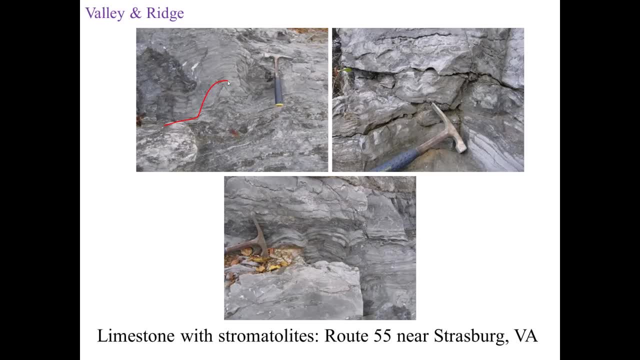 These are really cool carbonates that we see out on Route 55, and you can see they've got these neat structures in them called stromatolites, And stromatolites are sort of dome-shaped algal mats that grow upward. 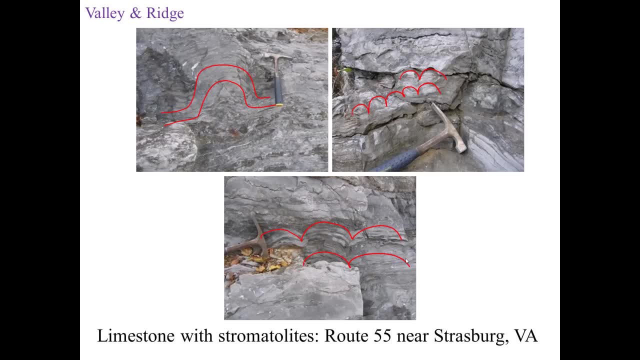 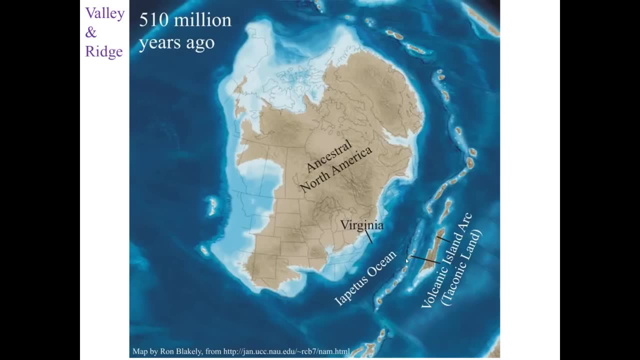 where we've got algae living in the limey water. So a look from a different angle, from outer space around 500 million years ago, would reveal something that looks more like this: We've got this Iapetus Ocean Basin that's opened up off the shore of North America. 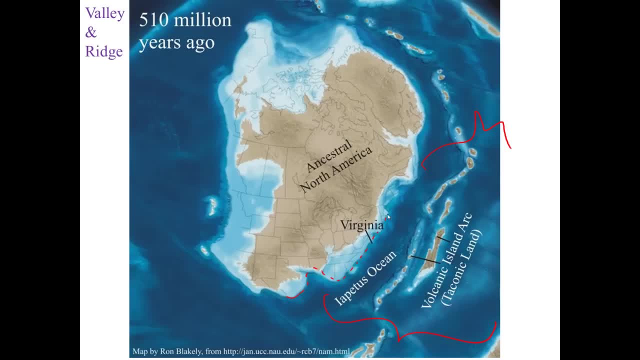 The edge of the North American continental crust is shown by the transition here between shallow water and deep water And you can see that part of Virginia here, the western part of Virginia, is present and basically accumulating these nice shallow water sediments, the ones that we just talked about. 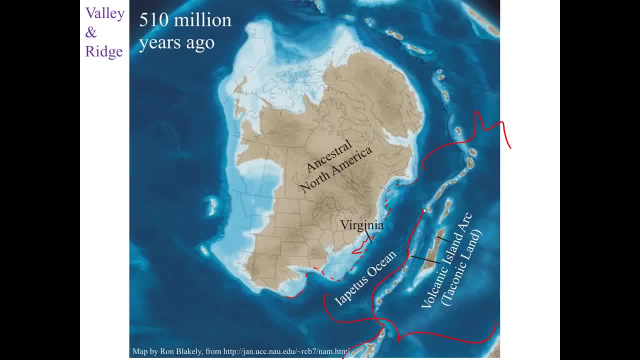 And on the shore in the Iapetus Ocean, you can see that the edge of the North American plate is getting closer and closer. There's a subduction zone and this oceanic crust is subjected to subduction. It's diving down underneath this plate of oceanic crust. 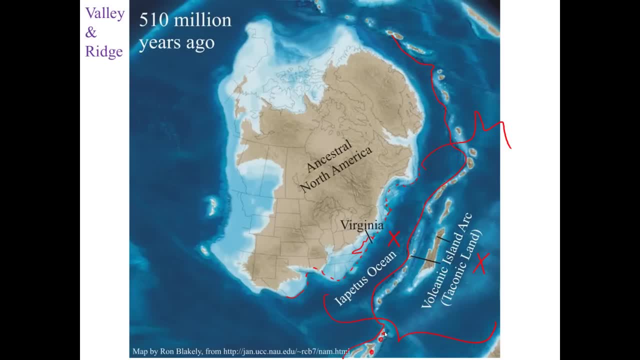 As it dives down, it experiences partial melting and some of that magma rises to the surface to erupt as a chain of volcanic islands, a volcanic island arc. That volcanic island arc is getting closer and closer to the edge of North America every day as this distance here is decreasing. 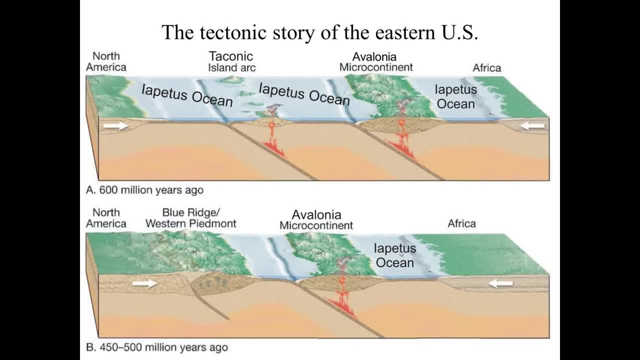 So the overall tectonic story of the East Coast during the Paleozoic era of geologic time is illustrated here. You start off with this situation in Virginia, like we've just talked about, but then you bring the oceanic crust on the edge of the North American plate. 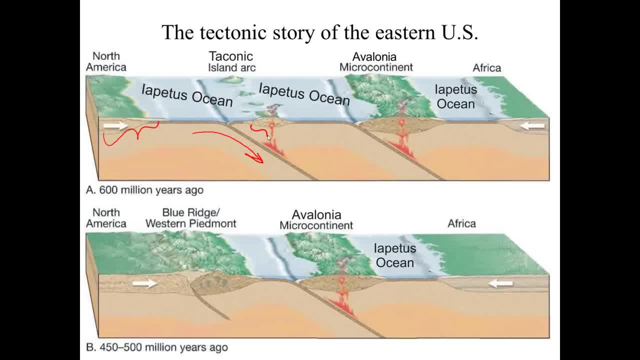 down into the mantle. That's a subduction zone, And so these volcanic islands are getting closer and closer And they're eventually going to run into ancestral North America. That's an episode of mountain building that takes place around 460 million years ago. 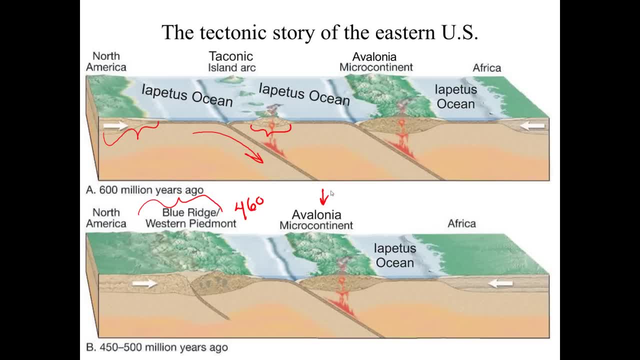 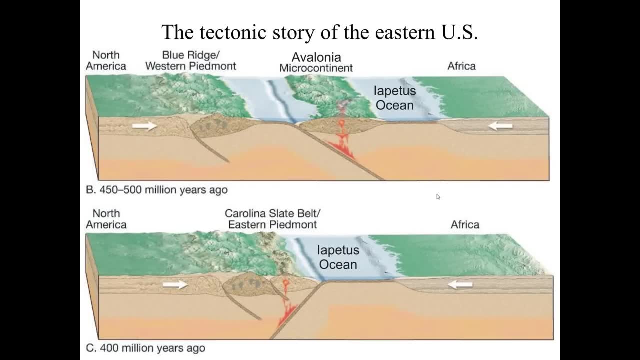 Meanwhile, there's a microcontinent out there in the Iapetus Ocean, and the other side of the Iapetus Ocean is the continent of Africa. As the Iapetus Ocean closes, that microcontinent called Avalonia also runs into the edge of North America. 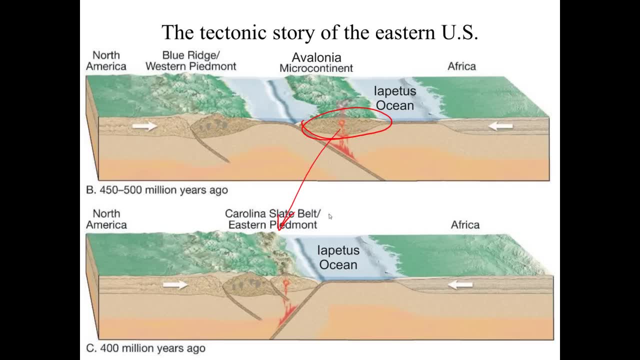 That's a second part of North America. There's a second period of mountain building, and that takes place more or less around 360 million years ago. a second orogeny, And then finally, we've got a little scrap of the Iapetus Ocean left. 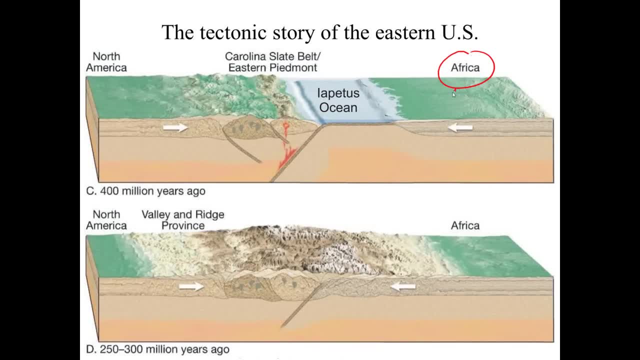 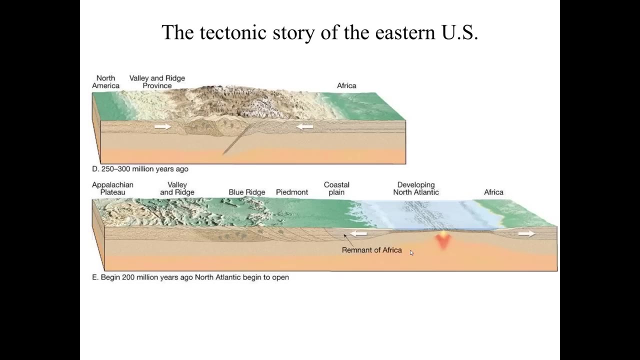 and that too will close, bringing Africa into direct collision with ancestral North America. And that raises up the young Appalachian Mountains, creates the supercontinent of Pangaea, and that is the death knell of the Iapetus Ocean. Pangaea, of course, doesn't last forever. 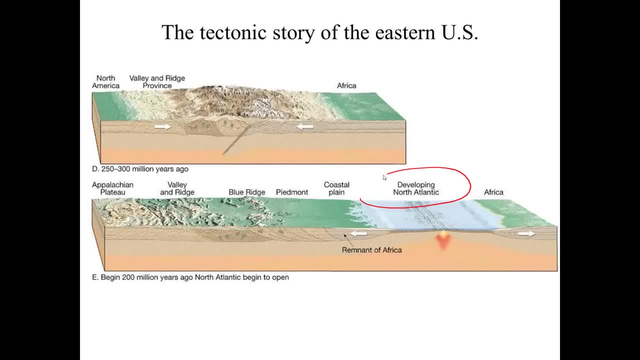 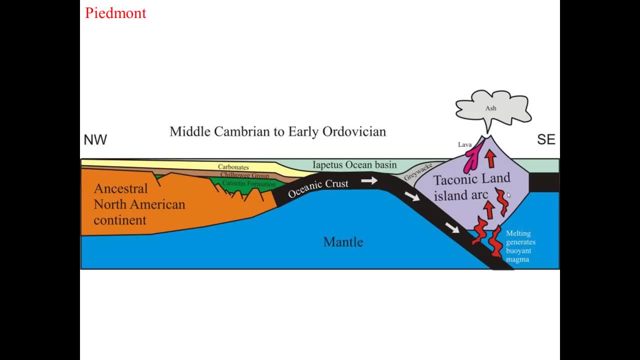 It breaks apart over time. and when it rifts apart, we open up the Atlantic Ocean between North America and Africa, which is now pulling away in the opposite direction. So let's take a look at the various pieces of this puzzle, one at a time. 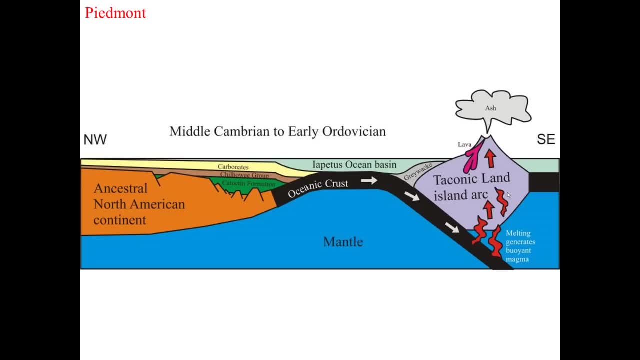 First is the collision of North America with this volcanic island arc. Here's a cross-section showing the volcanic island arc where it's erupting ash into the atmosphere, lava down the flanks of the volcanoes right there and then sediment such as graywacke. 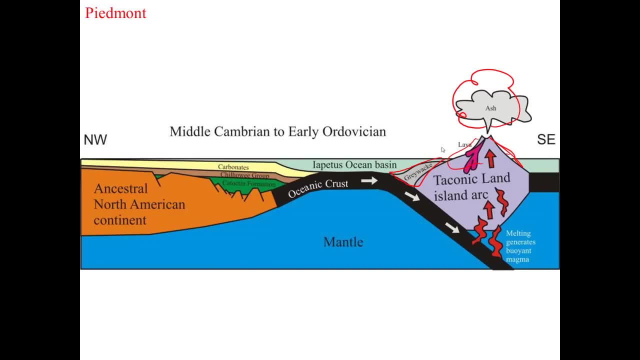 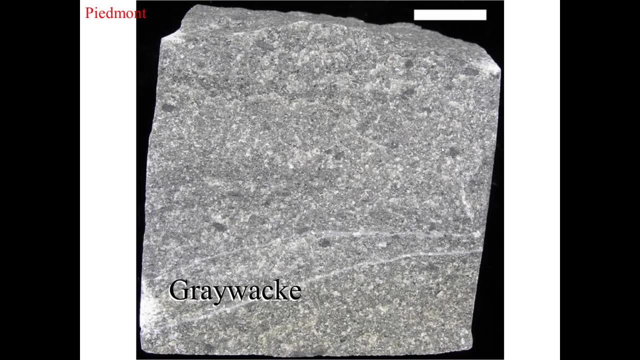 a dirty sandstone are being avalanched off into the Iapetus Ocean basin. Graywacke looks like this: It's basically a dark gray colored sandstone, a mix of sand and dark mud. It's deposited by so-called turbidity currents. 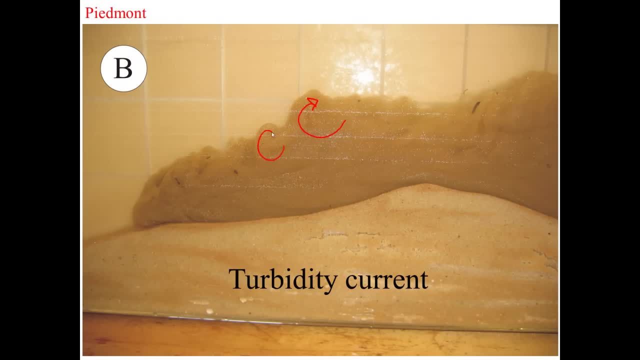 They're turbid because basically they are all complex, so they've got lots of little roiling currents in them that are keeping sediment suspended And as they go avalanching down the deep because they are dense, they carry all that sediment, big and small, with them. 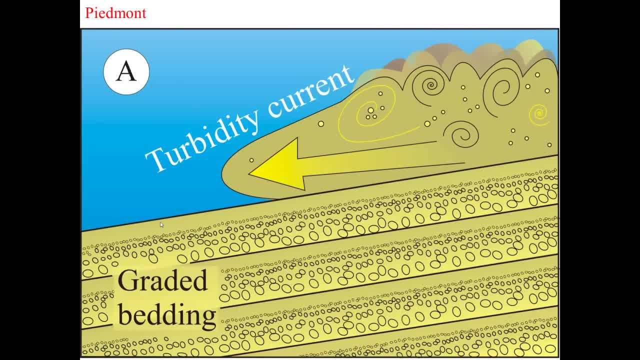 As they slow down, the big stuff settles out first and the small stuff settles out last. This produces a characteristic geological structure known as graded bedding. Graded beds are coarse at the bottom and then they get finer as you go towards the top. 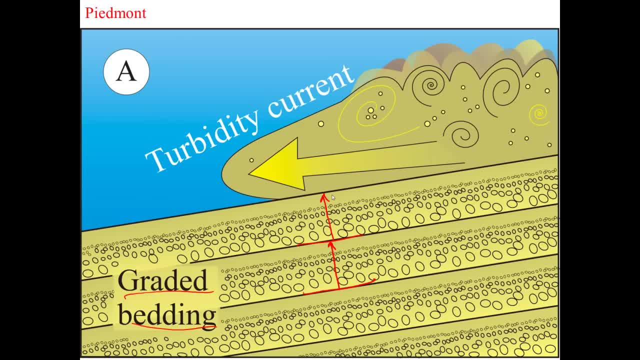 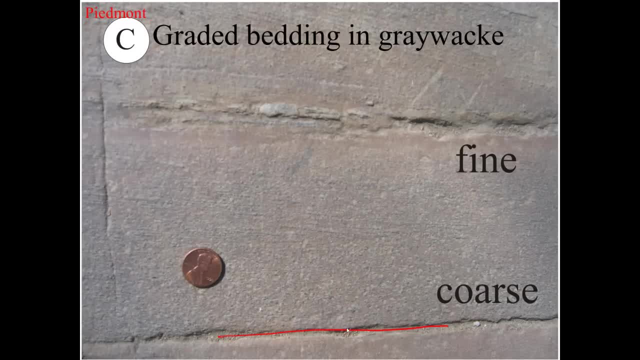 and then boom, you get a new graded bed which has that same coarse-defined pattern. Here's an example of graded bedding in metamorphosed graywacke from Great Falls Park, Virginia. There's the coarse bottom and then it gets finer towards the top. 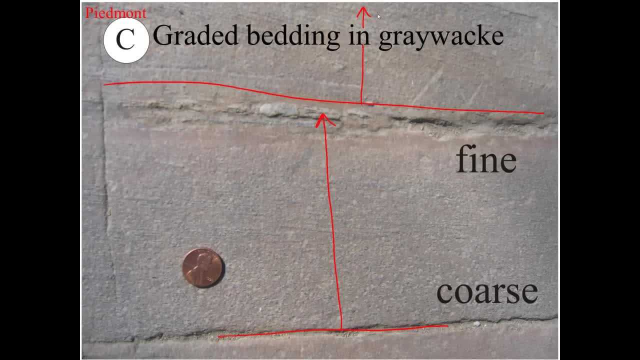 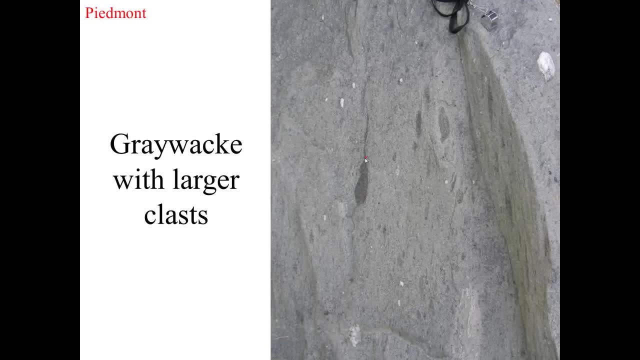 and there's another coarse there and it gets finer, going up again. Some of the graywacke in our area contains chunks of other rock clasts. Some of these clasts are dark in color, some are light in color, So these are particles of rock. 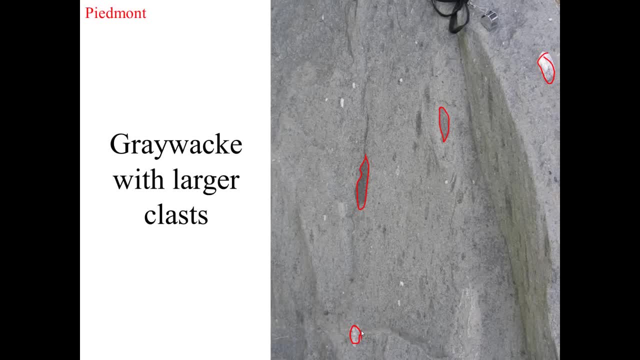 that predated the deposition of these sediments. So, whatever those rocks are, they come from older rocks than the deposit of graywacke itself. All of these sediments, these graywackes, mixed in with other stuff and not mixed in with other stuff. 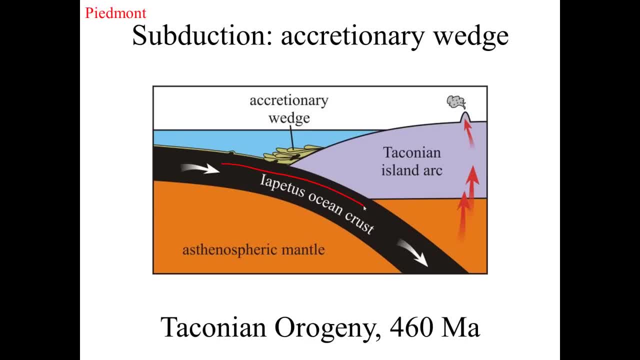 they get scraped off of the subducted plate. So, as this plate goes down the hatch here and produces magma that feeds the volcanoes, the sediments are being scraped off and they build up in a big pile called an accretionary wedge. 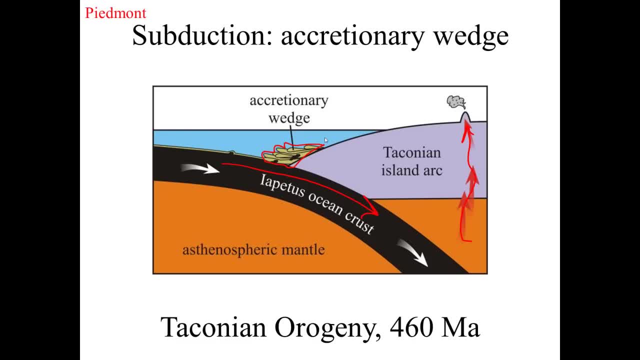 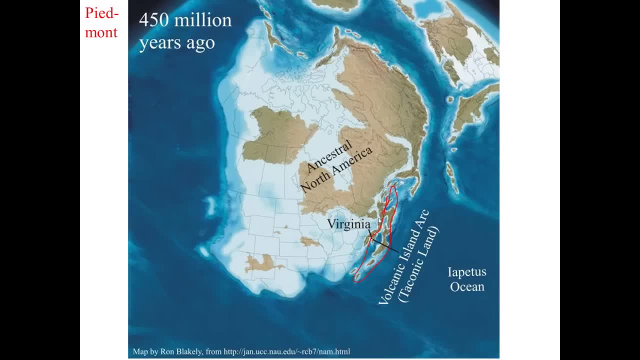 That accretionary wedge is much of the material that we find in the modern-day Piedmont Province. So as those volcanic islands crash into ancestral North America, mountains get raised, the crust crumples up and we end up getting metamorphism. 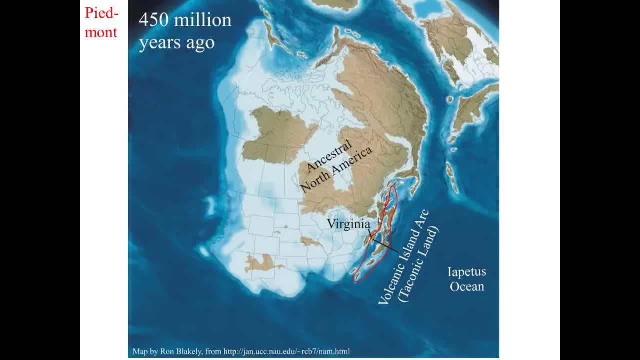 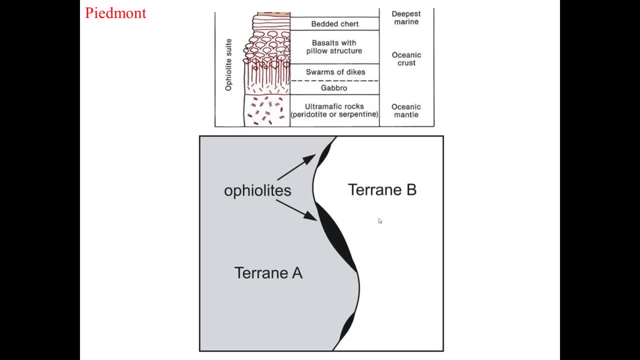 deformation and partial melting of those graywacke sediments in the accretionary wedge. So we also have little scraps of oceanic crust that get caught in between ancestral North America and the colliding volcanic islands. These little scraps of oceanic crust? 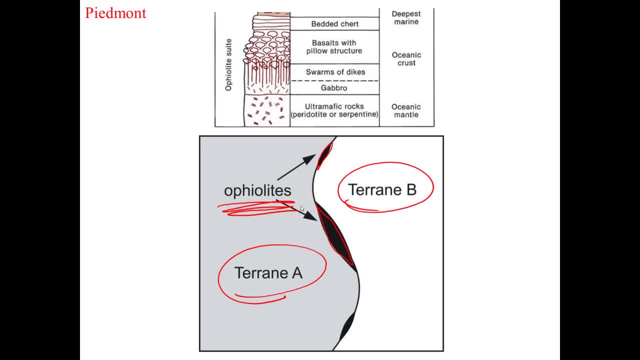 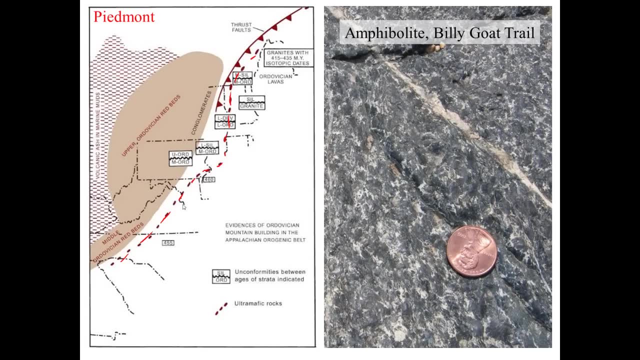 are known as ophiolites. So we've got a chain of ophiolites that runs up and down the East Coast, marking where the Iapetus Ocean used to be, and you can see that much of Virginia, for instance, is east of that line. 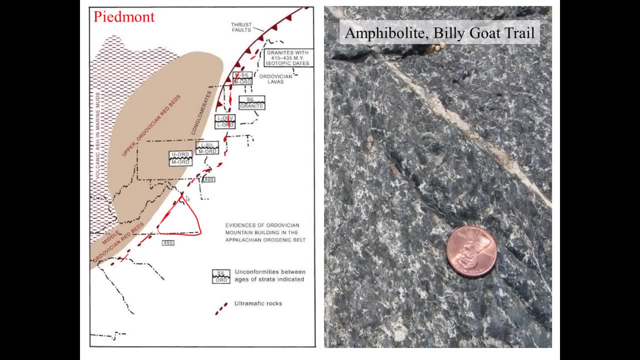 which indicates that that's new material that's been added on to Virginia. Some of the possible ophiolites in our area include amphibolite metamorphose basalt that we find along the Billy Goat Trail in Maryland. You can see these nice black lines. 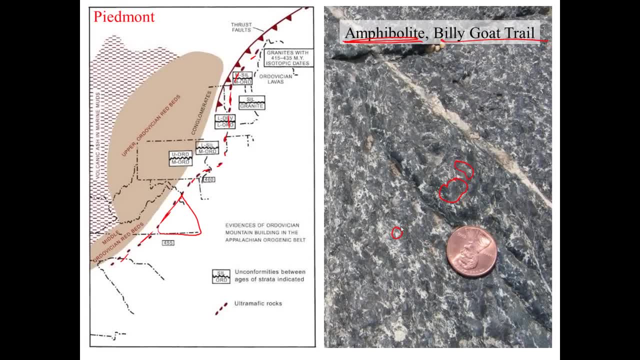 are the black crystals of amphibole there. The white stuff is plagioclase feldspar. We can see that our graded beds of graywacke have gotten folded. so deformation is something we associate with mountain building, and there's a nice example of that. 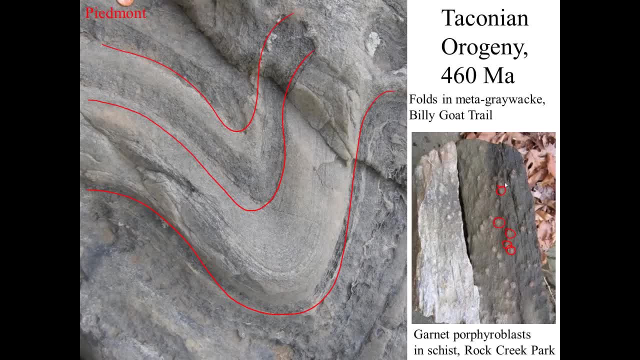 We also see metamorphism. Here are some garnets that have grown in a schist in Washington DC. Those garnets are not gem quality, but they do record high temperatures and high pressures experienced during this ancient episode of mountain building, the Toconian Orogeny. 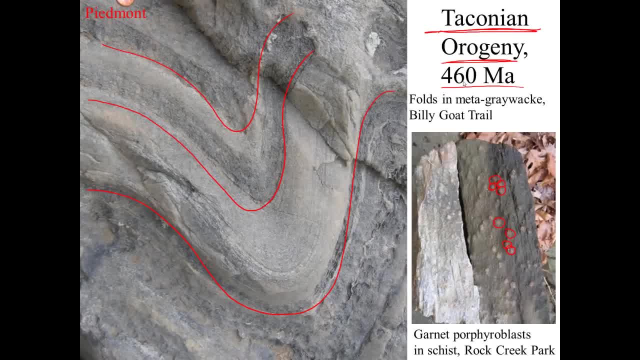 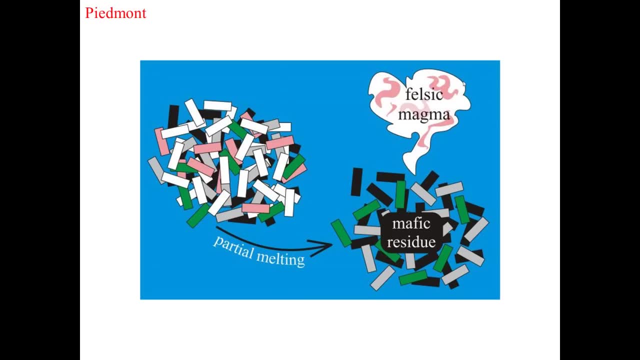 Again, that happened around 460 million years ago and it's called Toconian because it was first described up in the Taconic Mountains of upstate New York, One of the really nice aspects of the Toconian Orogeny in our area. 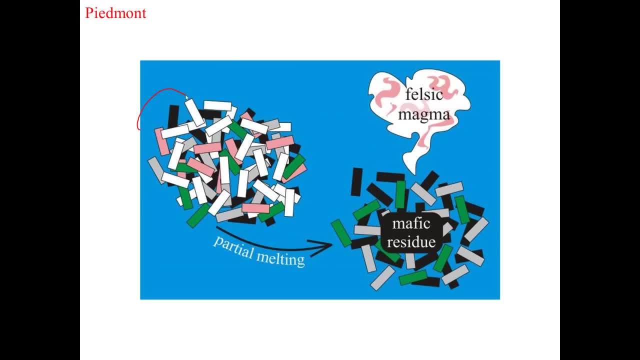 right along the valley of the Potomac River is that our original graywacke got melted. It didn't get completely melted, but it got partially melted, and that encouraged the minerals with the lowest melting temperature to separate out from minerals with higher melting temperatures. 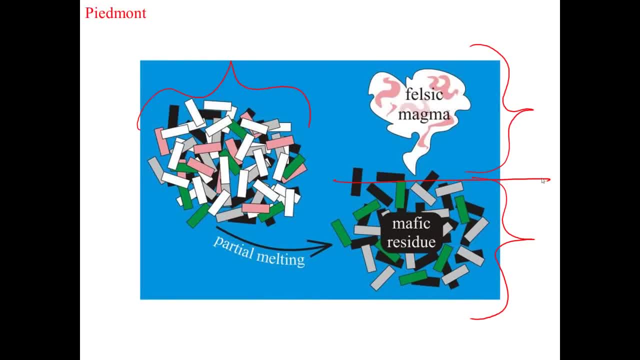 So, basically, it got hot enough to melt some, but not all, and so it melted out the felsic minerals, things like quartz, potassium, feldspar, muscovite, mica- and it left behind the mafic minerals. 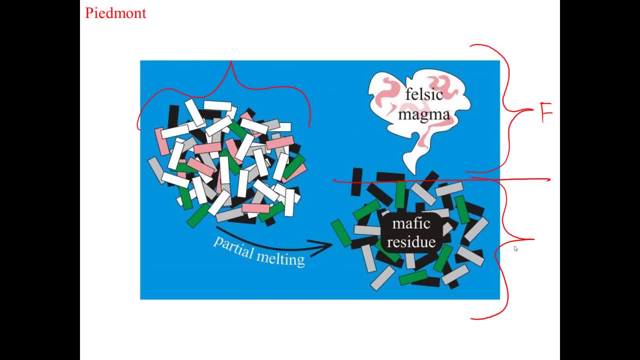 things like biotite, mica, amphibole and stuff like that. So the rock that shows visible textural evidence of partial melting is called a mygmatite. Mygmatite's very well exposed along the Billy Goat Trail. You can see here basically these little blebs. 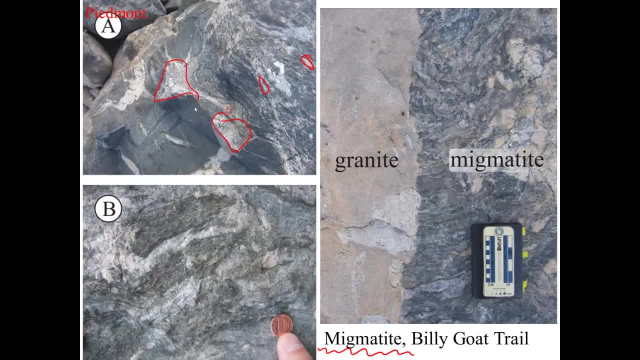 and blobs of granite that are coalescing to make larger bodies of granite. But in many places along the Billy Goat Trail you still have the little source, blebs and blobs. So that's a rock. that's sort of on the threshold between igneous and metamorphic. 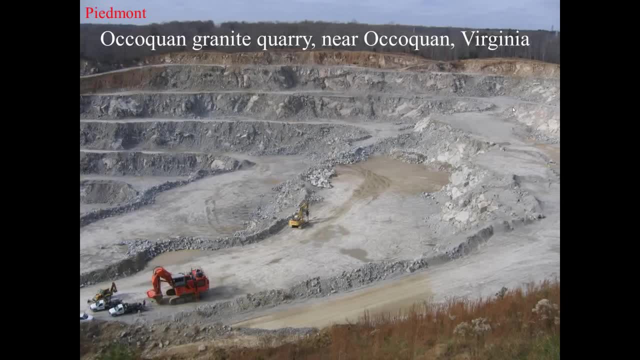 If the blobs get big enough, they can intrude as very big plutons of granite. So here's a pickup truck and some people to give you a sense of scale here. Everything you see in this picture is all granite, and all that granite is from the Toconian Orogeny. 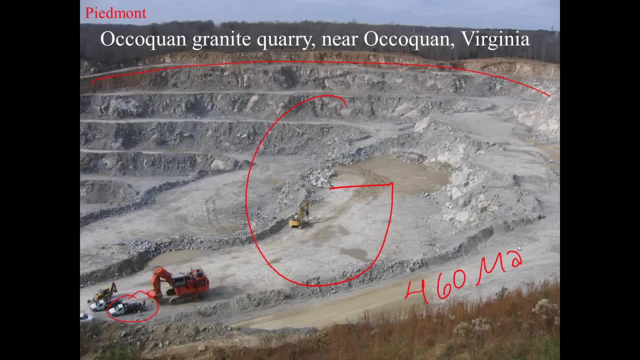 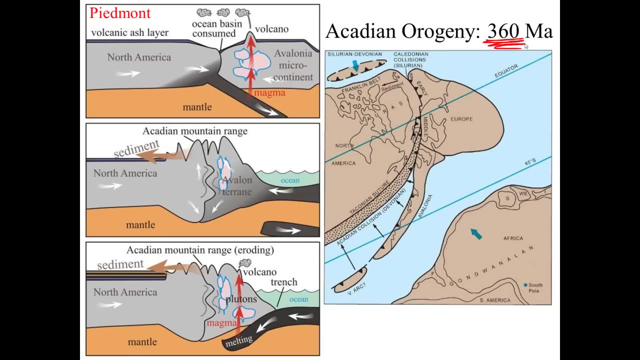 around 400 and something Around 460 million years ago. The Acadian Orogeny was the name for the episode of mountain building. that happened 360 million years ago, So that's 100 million years later after the Toconian Orogeny. 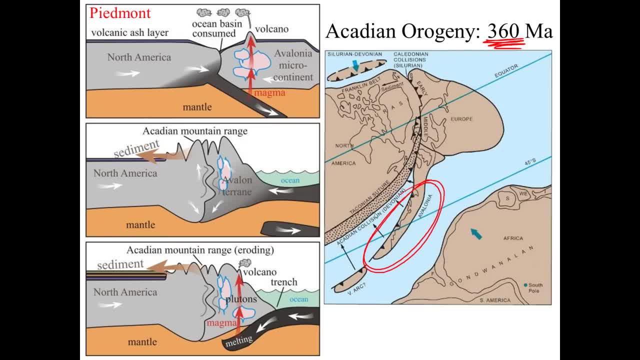 And that's due to this collision of a microcontinent called Avalonia with ancestral North America. As Avalonia collided, it built up a tremendous mountain range. That mountain range was a source of sediment and that sediment went coursing off towards the west. 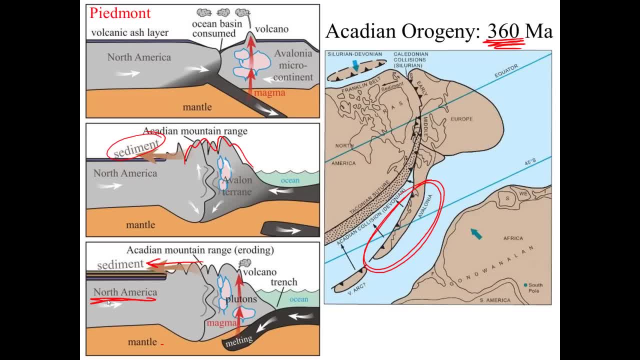 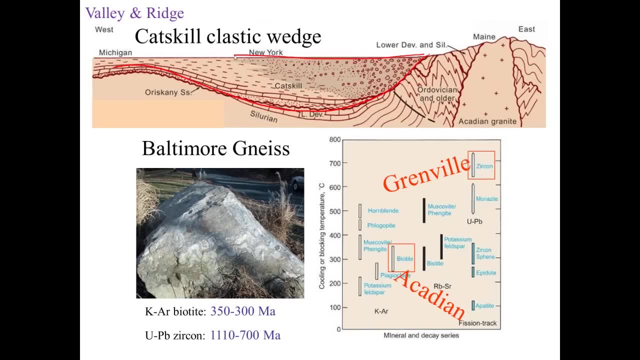 to be deposited on the un-mountainous interior of the North American continent, So that sediment looks something like this: There's a tremendous wedge of this sediment that came off the Acadian Orogeny. It's called the Catskill Clastic Wedge. 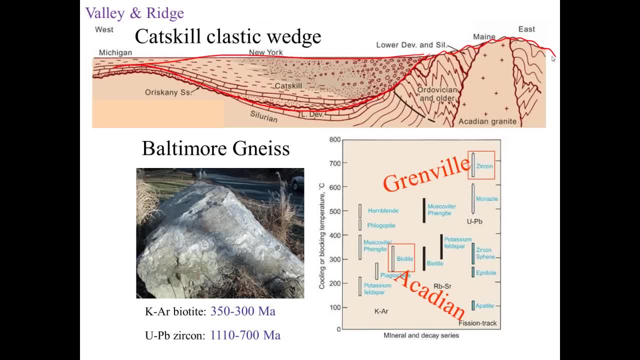 The mountain belt itself doesn't have any sediment from the mountain belt because that was a high area, then It was a source of sediments, not a low area where sediments accumulate, But at the roots of the mountain belt itself you'll find things like granite. 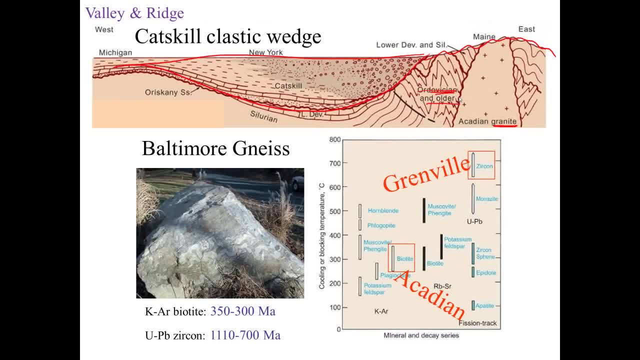 and then folded and faulted metamorphosis, So that's why it's called the Catskill Clastic Wedge, The sedimentary rocks, the Catskill Clastic Wedge. they tend to be coarse close to the mountain belt and then get finer and finer and thinner and thinner. 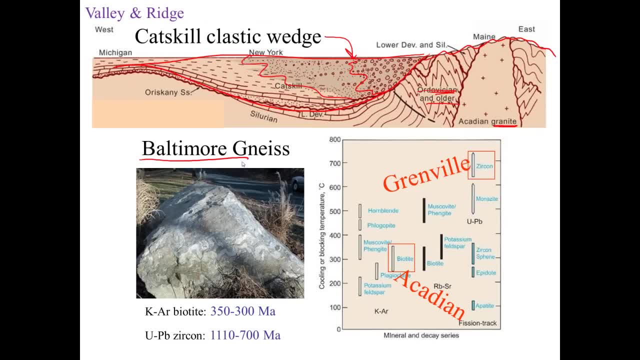 as you head towards the west. In Baltimore, Maryland, we have an interesting rock called the Baltimore Gneiss. The Baltimore Gneiss has two different dates that it'll give you two different isotopic ages If you do uranium lead dating on zircon. 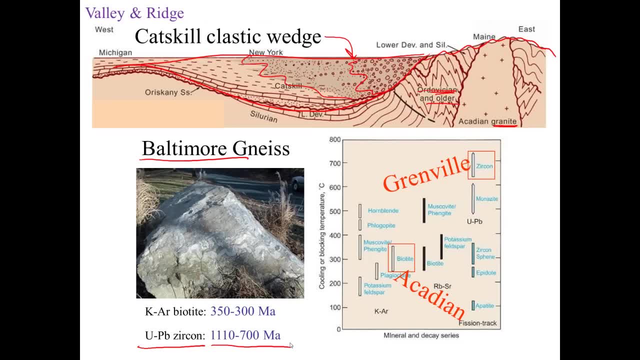 it gives you an age of around 1.1 billion years. If you do potassium argon dating on biotite, it gives you an age that's around 350 million years old. So what that tells you is basically: the biotite age has been reset. 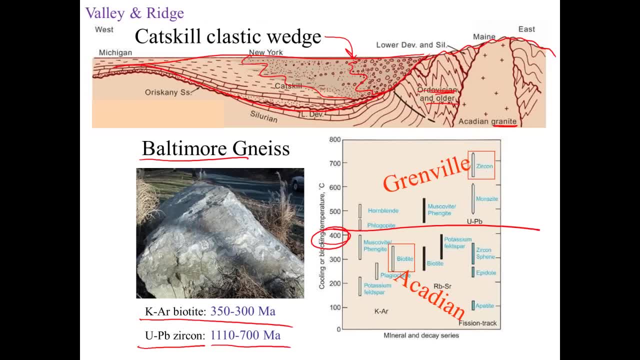 This rock must have gotten heated up to maybe 400 degrees, something like that. That's enough to reset the biotite age and give you the metamorphic age of the Acadian orogeny, but not hot enough to reset the uranium lead date. 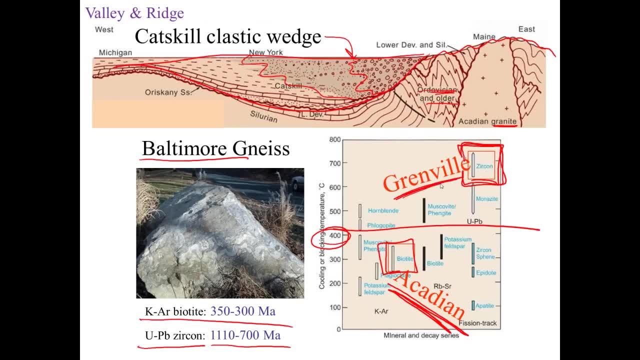 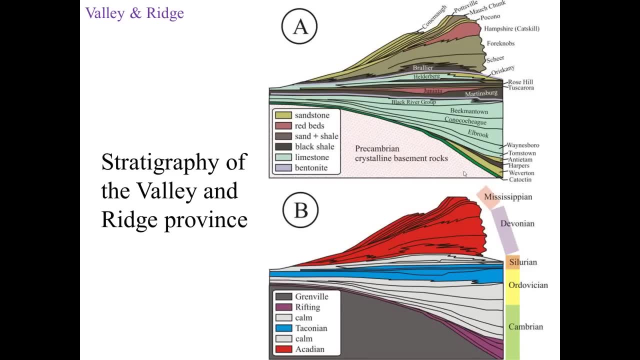 that's hidden in the zircon crystals. That gives you the Gneiss' original age, which is Grenvillian. Let's take a look now at the valley and ridge province. This is what it would look like if we unfolded and unfaulted. 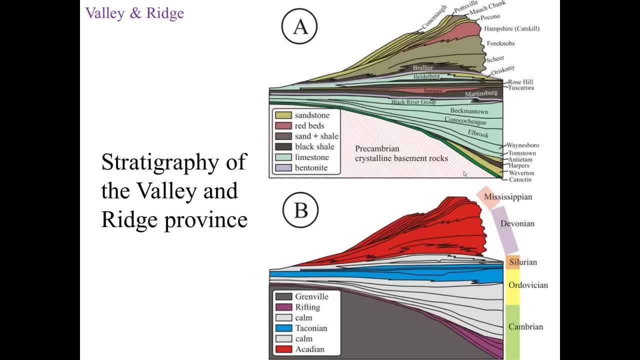 all of those sedimentary layers that make up the western Appalachian Mountains. You can see here that it's a big, complex stack. A couple of patterns will jump out. If you look at the upper figure first, you'll notice that it is much thicker in the east. 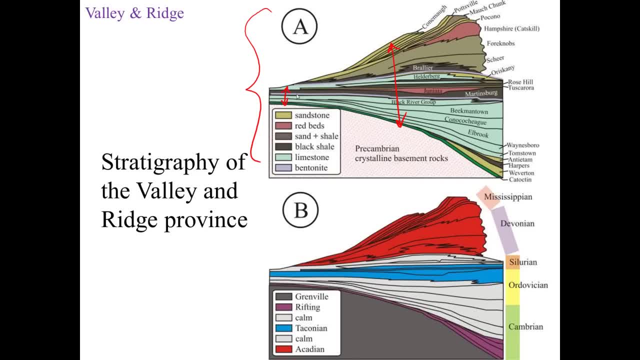 than it is in the west. So that probably has to do with being closer to the original mountain source for a lot of these sediments, And then also where the crust is right next to a mountain range, it tends to bow down, meaning that there's more room. 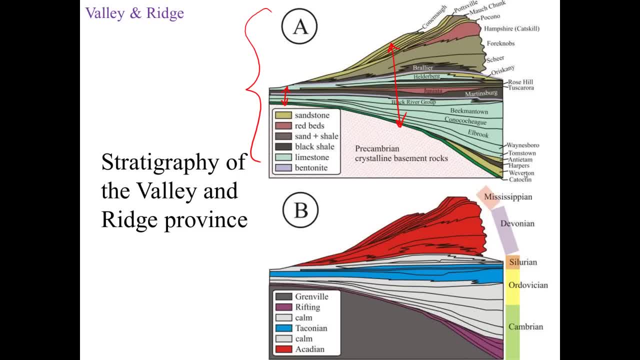 to accumulate sediments. If you wanted to not memorize the names of all these different formations- and why would you, unless you're going to be a sedimentary geologist- you can take a look at the lower picture, which basically summarizes what's going on here. 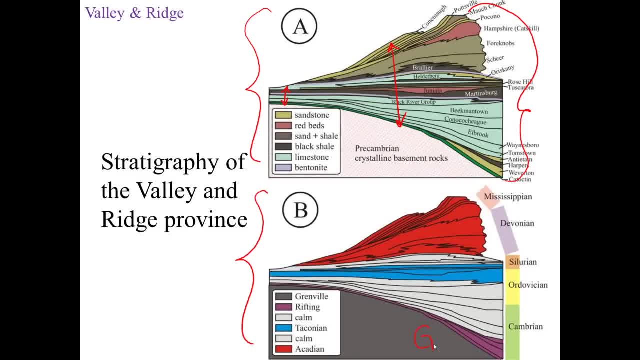 You've got these Grenvillian Age basement rocks. then you've got these rift-related rocks where the Iapetus Ocean was opening up. Then you have passive margin sediments from the tectonic calm between the rifting and the Toconian Orogeny. 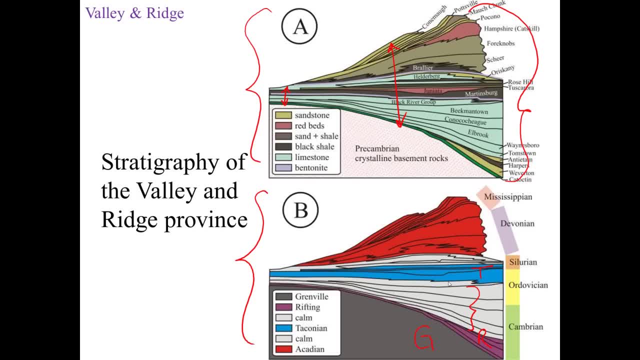 The Toconian Orogeny. those mountains produced a lot of sediments which give you that sort of dirty package there in the middle. Then you have another period of passive margin sedimentation before the Acadian Orogeny hits, And then all this red stuff up at the top. 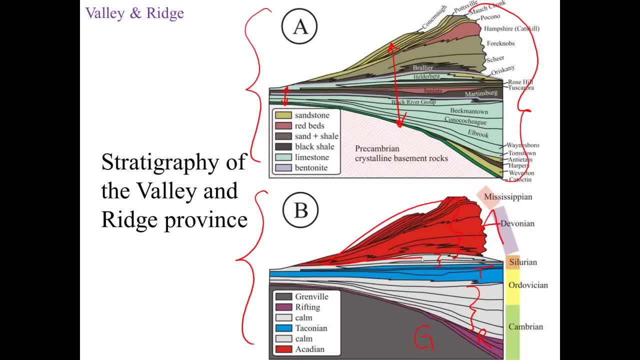 that's from the Acadian Orogeny. So if you just look at the amount of stuff that came off the Acadian Orogeny and compare it to the amount of stuff that came off the Toconian Orogeny, you can see the Acadian Orogeny must have been. 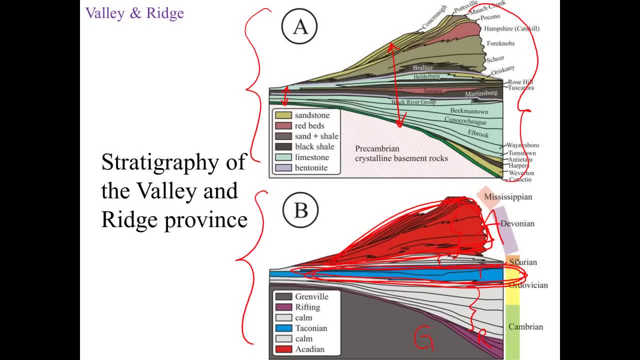 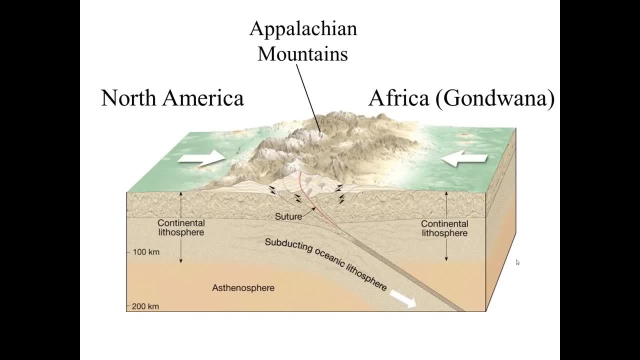 a bigger mountain building event, because it basically spewed a lot more sediment into the low-lying areas to the west. The final episode of mountain building that occurred in Virginia during the Paleozoic was the Alleghenian Orogeny. This is when ancestral North America 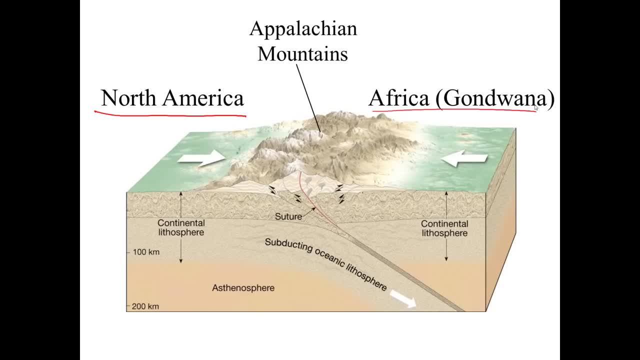 collided with ancestral Africa, which was the leading edge of the Gondwanan supercontinent at that time. The collision between the two raised the young Appalachian Mountains, which probably would have been Himalayan in extent. The suture there between them marks the little sliver that used to be the Iapetus Ocean. 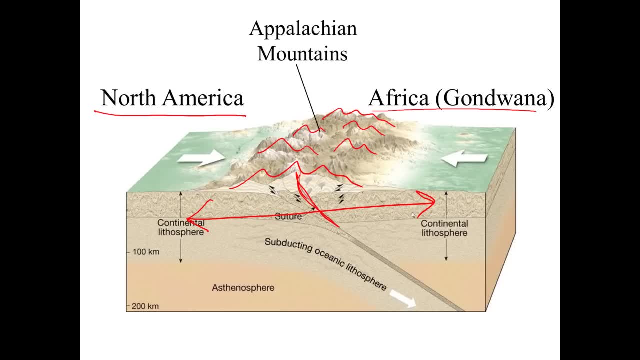 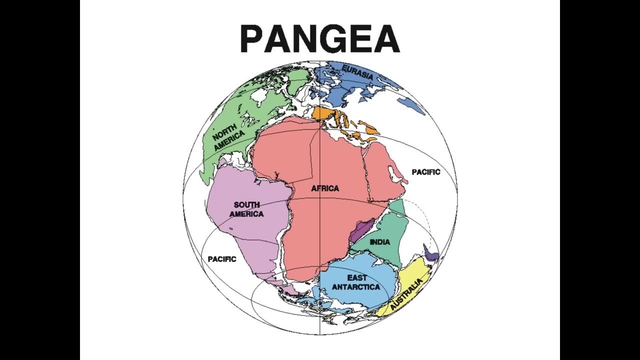 And, of course, now the connected two pieces of continents makes a new supercontinent, and that is the supercontinent Pangaea. Pangaea was the largest supercontinent ever known. We've been looking at this little zone right here, but there are plenty of other connections. 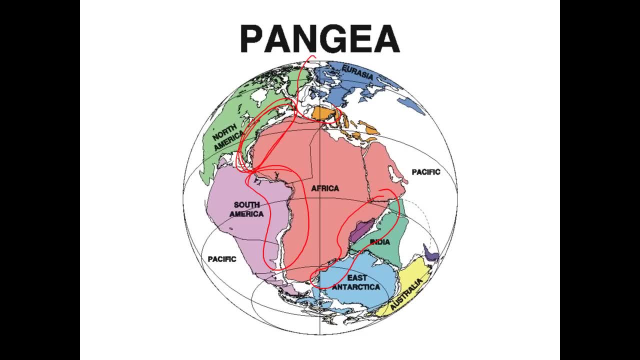 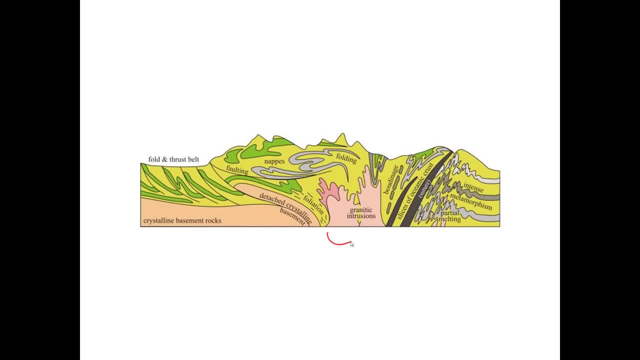 between different continental fragments all around the world. that helped to make Pangaea A cross-section through the young Appalachian Mountain Belt would show granite intrusions, ophiolites, partial melting, intense metamorphism. in the Piedmont Province It shows a detached chunk. 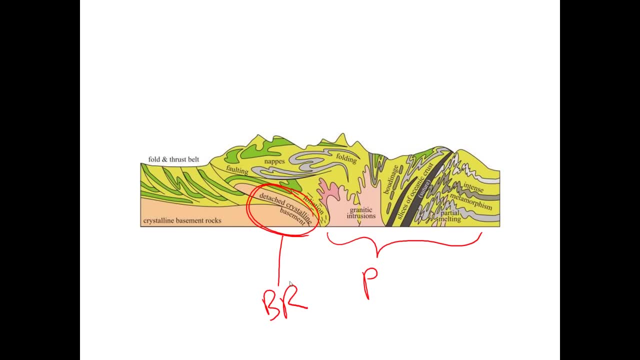 of crystalline basement. that's the Blue Ridge Province. And then we've got the folded and faulted sedimentary rocks. that's the Valley and Ridge Province. So zooming in on the Blue Ridge Province here you can see it's this sort of chunk. 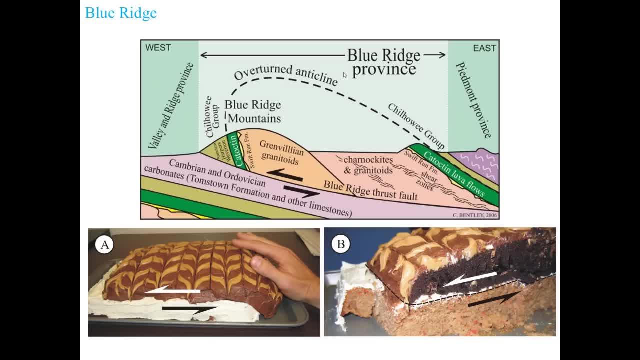 of the basement rock that has been bowed upward into an anticline. The rocks that you find in the western part of the Blue Ridge Province, in the Blue Ridge Mountains, match up with the rocks you find on the eastern part of the province And we think that probably at the bottom of the Blue Ridge. 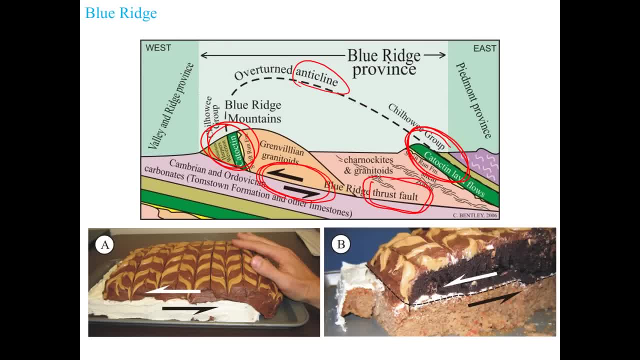 is a big thrust fault. So one way to explain that thrust fault is to think of a couple of cakes. Imagine that I baked a chocolate- peanut butter cake on Monday, so that's the older of the two cakes- And then I baked a carrot cake on Wednesday. 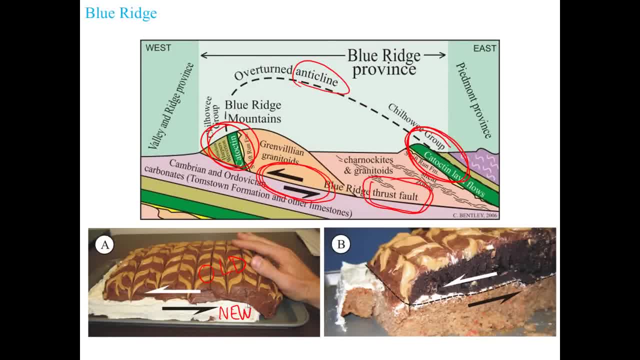 that's the newer of the two cakes. And then on Friday I shoved my old cake on top of my new cake And it traveled along this nice little greased layer of icing And came to rest with the older on top of the newer. 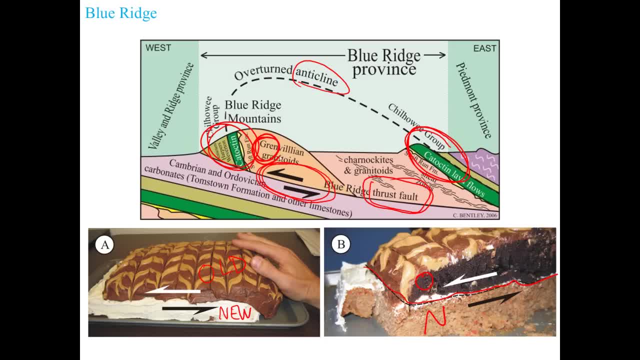 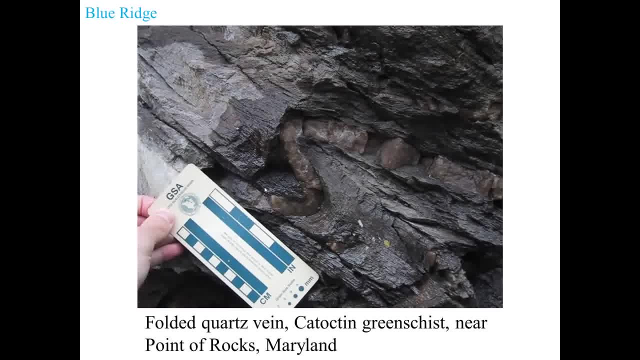 And that's the situation in the Blue Ridge, where you've got old rocks on top of relatively new rocks that are much younger. There was plenty of deformation that accompanied the Allegheny and Orogeny. Here is a quartz vein that has been folded. 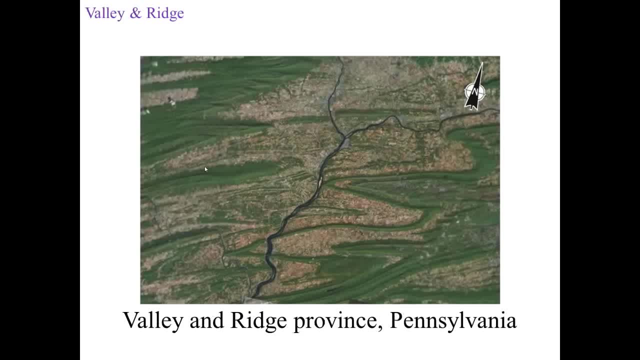 into a beautiful S shape. There's plenty of folding that takes place in the sedimentary layers as well. You can see here that there's a single sedimentary layer that's been folded all over the place. This is up in the Valley and Ridge Province of Pennsylvania. 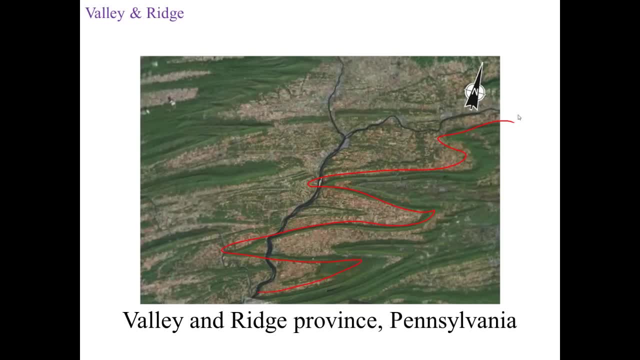 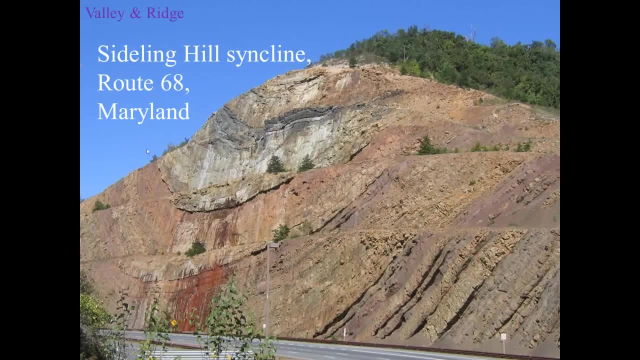 which for some reason they call the Ridge and Valley Province. A nice local example is on Interstate 68 near Hancock, Maryland, where the sedimentary layers of the Rockwell and the Purse Lane formation have been folded downward into an enormous syncline. 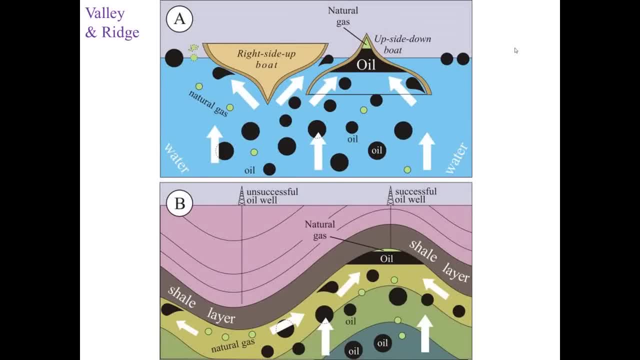 These anticlines and synclines are very important for our economy. You can think about their role in trapping oil and natural gas in the context of a couple of boats. If one of your boats is right side up and you release oil and gas into the water underneath, 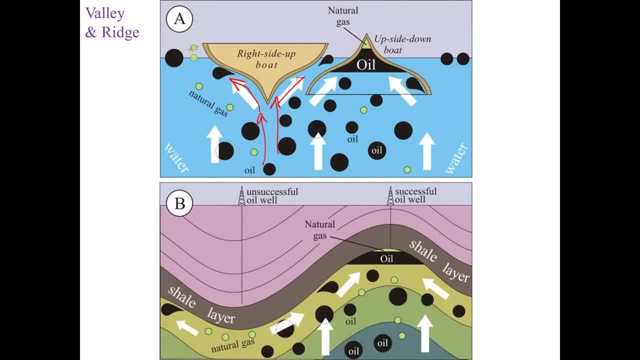 the oil and natural gas will rise up, basically hit the bottom of the boat and get diverted off to the sides to be released into the air. But if you have an upside down boat, any oil or natural gas that rises beneath it ends up basically being trapped. 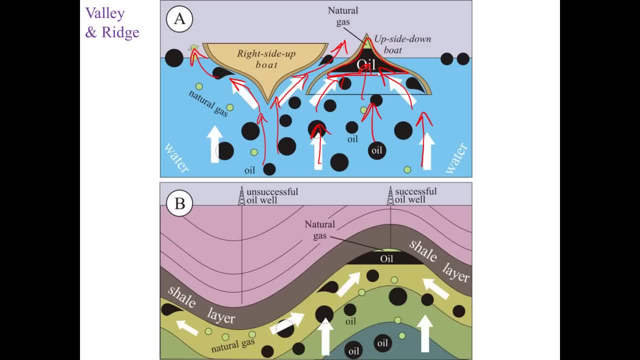 It can't get out, and so it tends to accumulate there in a little pocket. In the same way, impermeable rock layers that have been folded into synclines and anticlines have a similar role in diverting oil and natural gas in the subsurface. 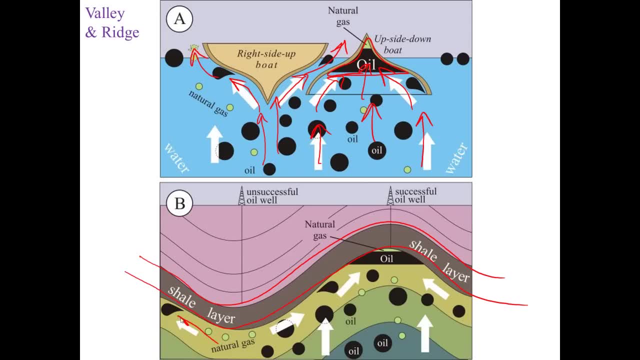 Synclines are a lousy spot to look for oil and natural gas because it gets diverted off to the sides, but anticlines are a great spot to look for it If you were a petroleum geologist and you told the oil company to drill this well. 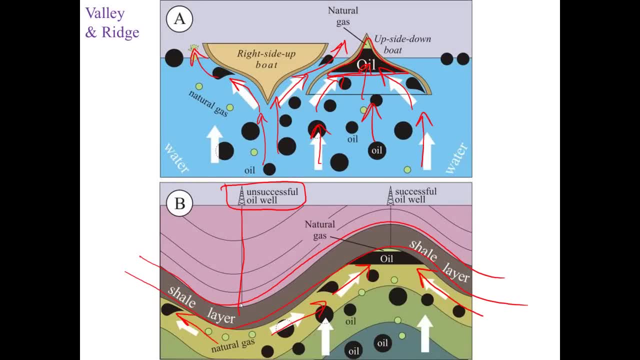 they would spend a lot of money drilling a very long well and they wouldn't get anything for their efforts, so you'd likely lose your job. On the other hand, if you could spot the anticline, you could tell them to drill this well instead. 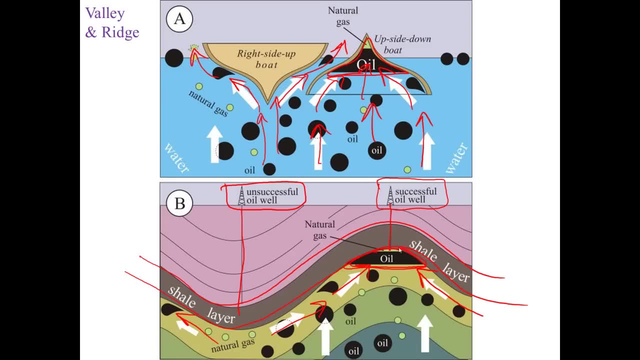 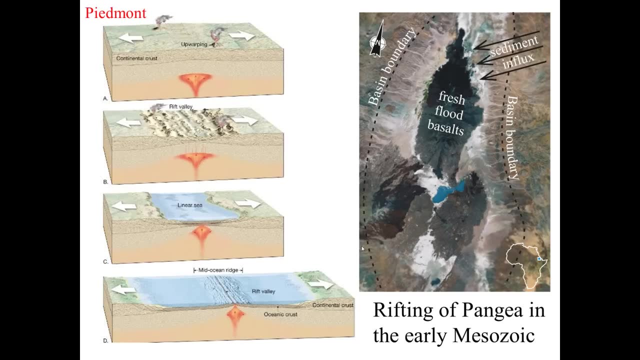 which is relatively short and taps into a nice pocket of oil and natural gas. All right, let's briefly now talk about the rifting of Pangea. We talked earlier about how Rodinia broke apart and it made the Iapetus Ocean. 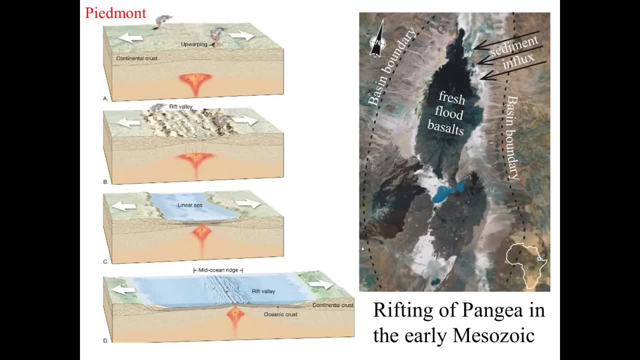 Now Pangea is going to break apart and it's going to make the Atlantic Ocean. The same sort of pattern prevails, where we end up getting rifting, normal faulting and volcanism that opens up into a linear sea and then that linear sea widens and widens over time. 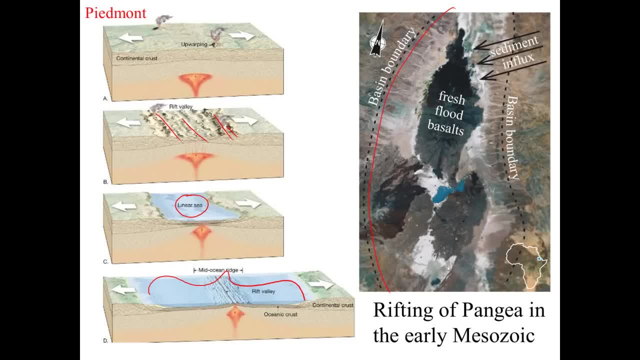 through seafloor spreading, So we end up getting a new series of rift valleys with a new influx of sediment and new eruptions of mafic lava. It's just like what we saw when Rodinia broke apart. This time, the rift basins are a little bit better exposed. 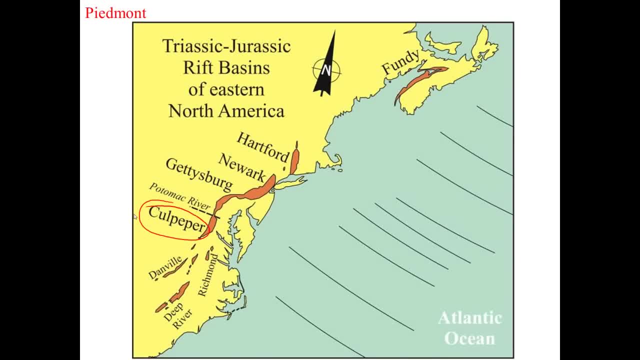 The big one that we have in Virginia is called the Culpeper Basin, But we've got lots of little ones in Virginia as well. There are other rift basins that go up through Gettysburg, Newark, New Jersey, Hartford, Connecticut. 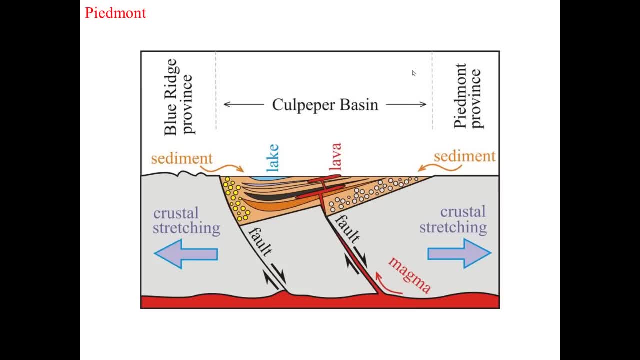 and even the Bay of Fundy up in Canada. If you do a cross section through the Culpeper Basin, this is what you'll find. You'll see Blue Ridge rocks to the west of the Culpeper Basin, metamorphic Piedmont rocks to the east. 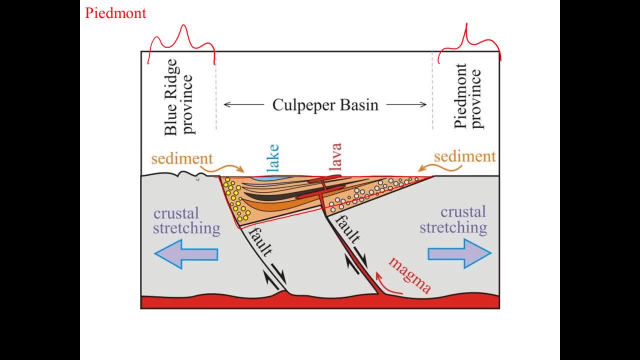 Then the Culpeper Basin itself is sort of shaped like a triangle. It's got coarse sediments along its edges. These are conglomerates. It's got fine-grained sediments deposited in lakes in its middle And then some of the faults that broke there. 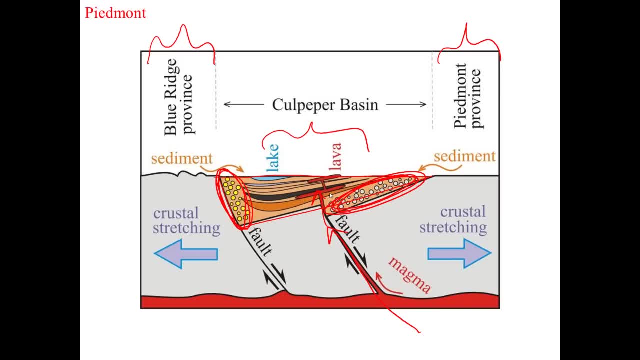 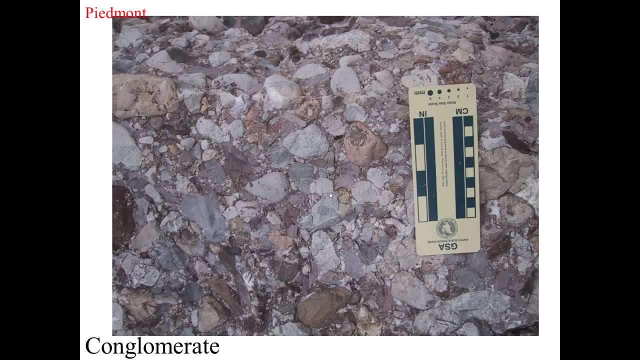 allowed magma to come up, and that magma is mafic igneous rock today. Here's a look at one of the coarse-grained rocks along the edges of the Culpeper Basin. This is the Leesburg Conglomerate, a conglomerate made out of pebbles of limestone. 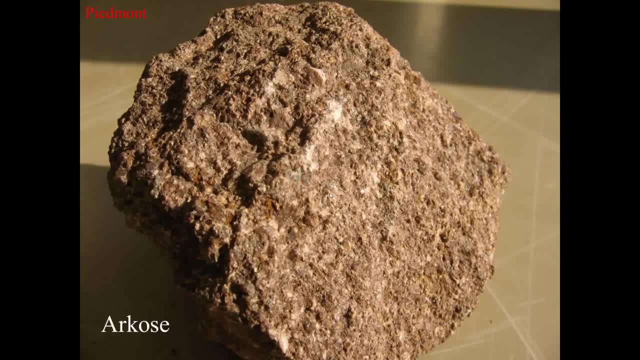 We also get sandstones, in particular the sandstone called Arcos- that's characterized by lots of potassium feldspar- big angular potassium feldspar grains in it, telling you it's not very mature. This is sand that was deposited only a few miles from wherever it started off. 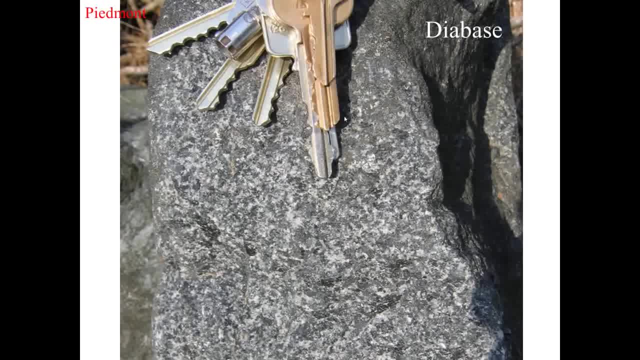 The mafic igneous rock that is left in the Culpeper Basin today is actually not an extrusive igneous rock, a basalt, but a slightly below-the-surface mafic igneous rock called diabase. You can see here with some keys for scale: 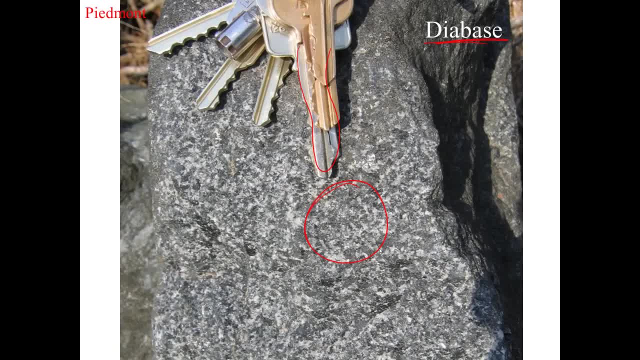 that this diabase does have crystals that you can see with the naked eye. So it's not as fine-grained as a basalt, but it's not really as coarse-grained as a gabbro. So diabase is essentially the same composition. 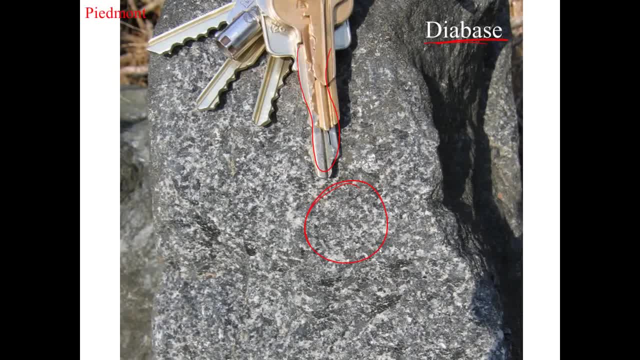 as a gabbro or a basalt, but its texture is sort of midway in between the two. Diabase is widely quarried in the Culpeper Basin for use as gravel and riprap. Some of the sandstone in the Culpeper Basin. 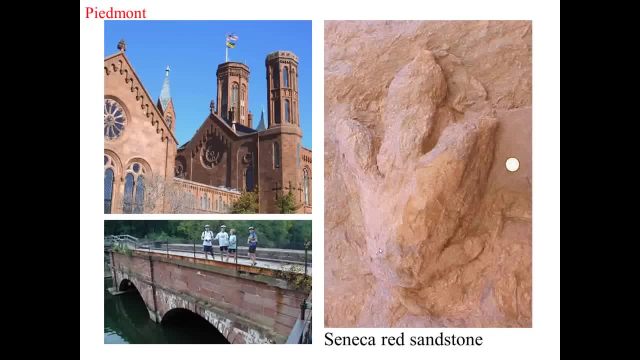 is a bright, beautiful red in color. It's called the Seneca red sandstone. It was used to build the locks and the aqueducts along the C&O Canal. It's also the Smithsonian Castle down on the National Mall. In places, the Seneca red sandstone. 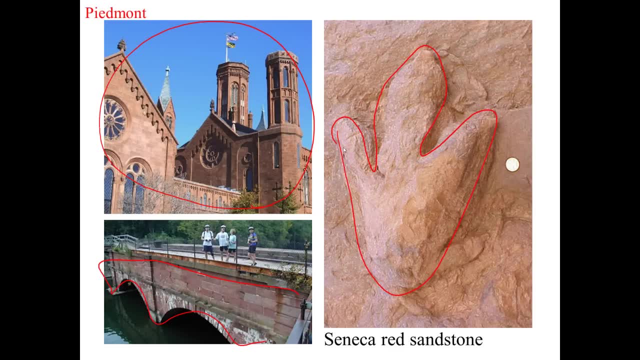 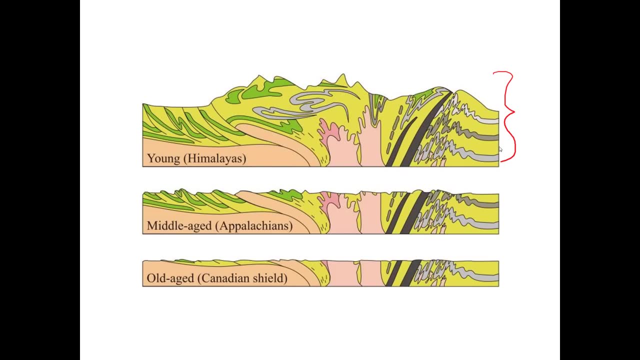 holds trace fossils of dinosaurs. Then the landscape was weathered away and the young Appalachian Mountains, which were awesome and Himalayan in extent, got worn down to their modern-day middle-aged version, and they'll continue to wear down in the future. 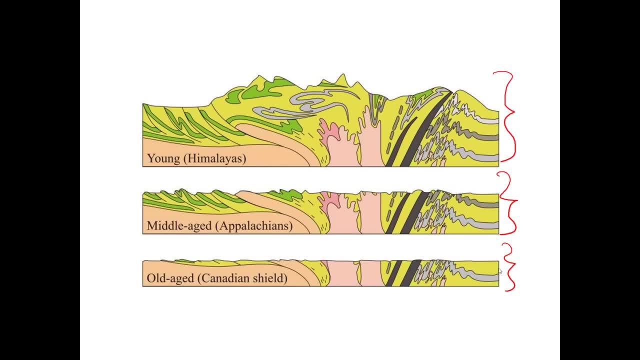 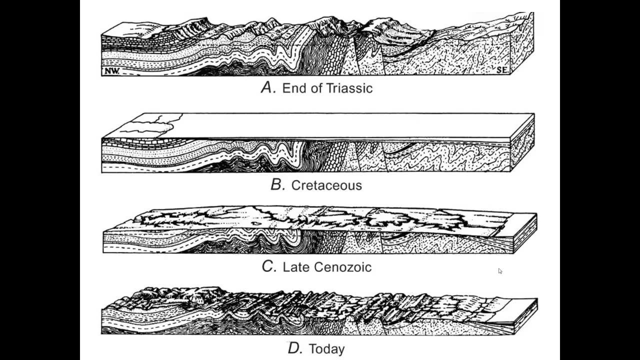 until they're not mountainous at all, and they'll look like the old mountain belts that crisscrossed the Canadian Shield. One interesting wrinkle on this story looks like the Appalachian Mountains were essentially worn down to a flat level by the Cretaceous period of geologic time. 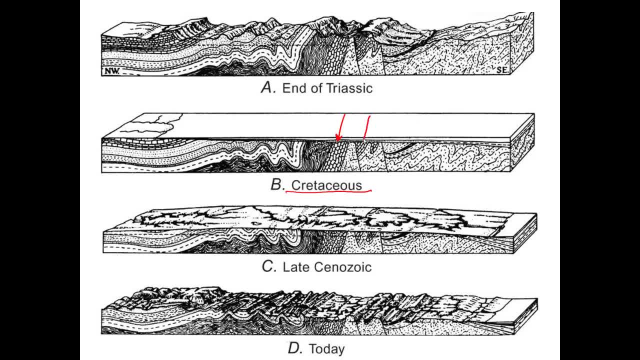 We know this because at that point the rivers stopped cutting down and they started depositing new layers of sediment on top of the eroded roots of the Appalachian Mountains. But after the Cretaceous, the rivers started to cut down in again, and so they incised new river valleys. 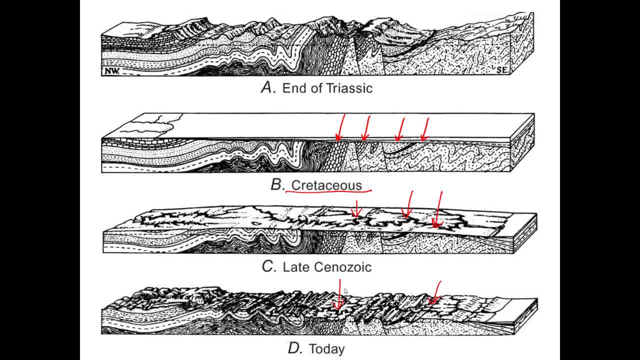 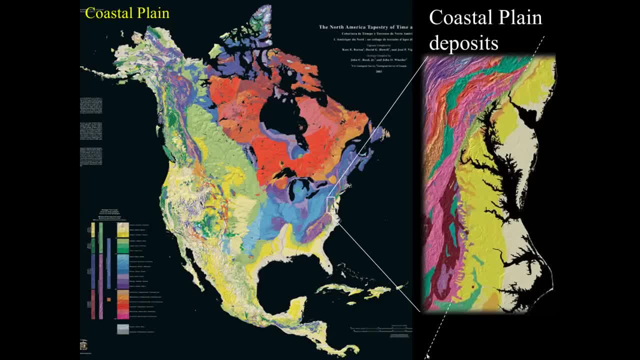 and those river valleys basically etched the landscape out into high relief once again. The youngest rocks in Virginia are the rocks of the Coastal Plain. The Coastal Plain rocks are located basically east of the boundary with the Piedmont rocks. They include rocks that are both. 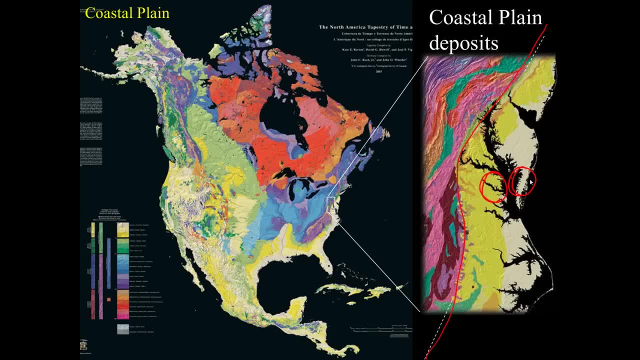 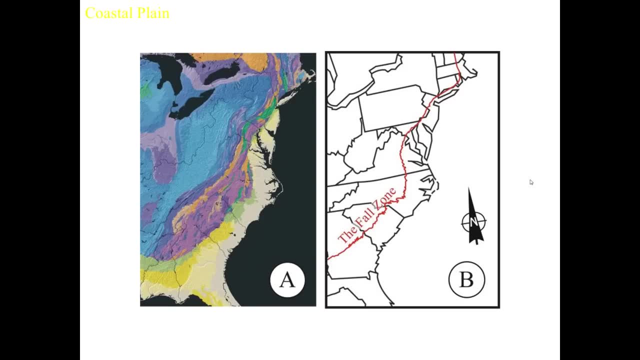 west and east of Chesapeake Bay and the boundary between the Piedmont and the Coastal Plain is known as the Fall Zone. Basically, any rivers that drain across that Fall Zone have waterfalls right there where they cross that particular line. If you were a colonist from Europe, 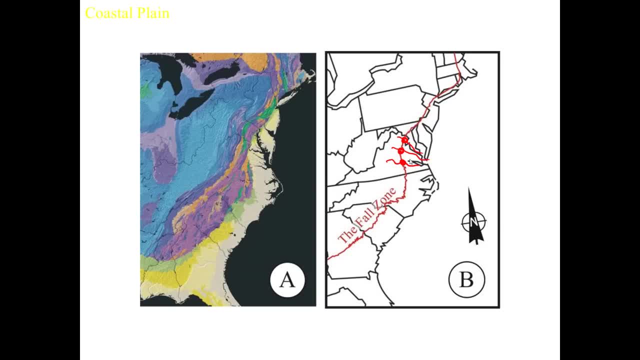 say, San Francisco, sailing up the Potomac River, the York River, the James River, back in the early days when North America was being colonized, you would start running into rapids and waterfalls right when you crossed that boundary. A cross-sectional view of the Fall Line. 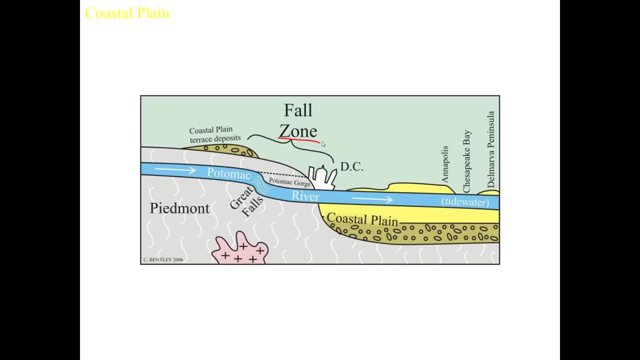 more properly known as the Fall Zone, is shown here. You can see those Cretaceous-aged gravel deposits that we mentioned earlier, deposited on top of the eroded roots of the Piedmont, and then the waterfalls started off where today you find Georgetown, in Washington DC. 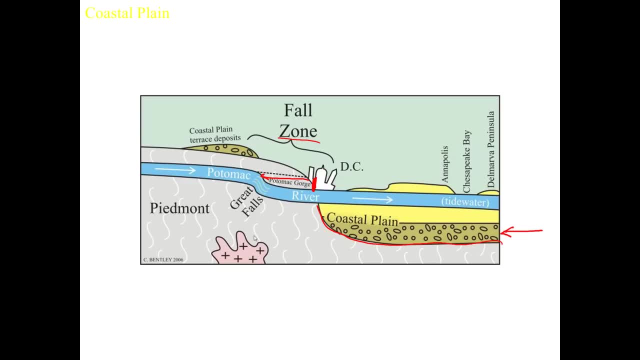 Since that time, though, the waterfall has moved upstream and can be found today at Great Falls, on the boundary between Maryland and Virginia, and the Potomac Gorge is in its wake. This is what those Cretaceous-aged river gravels look like. 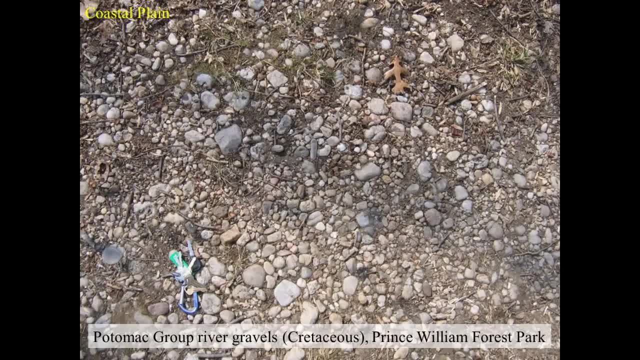 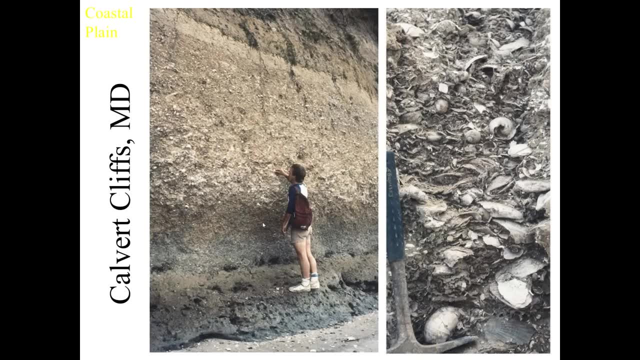 Fairly mature sediments, well-rounded, quartz-rich, but very coarse-grained. Higher up in the stack of sedimentary rocks in the coastal plain you can find Miocene-aged layers like those exposed at Calvert Cliffs, Maryland. These are composed almost entirely of fossils. 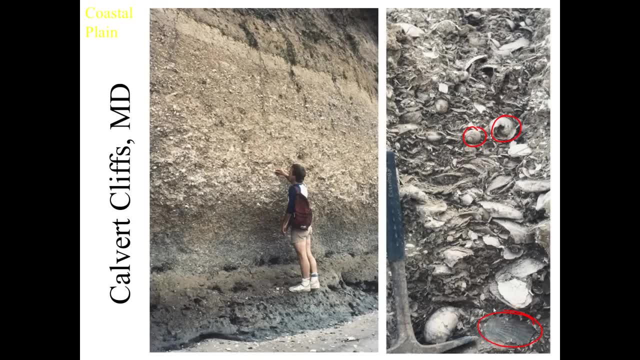 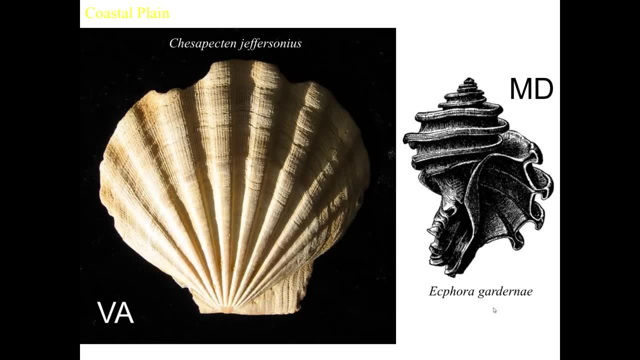 You can see things like snails and scallops in there, and you can even find really giant shark teeth. The state fossils of both Virginia and Maryland come from the coastal plain. Virginia's state fossil is a scallop known as Chesapectin jeffersonius. 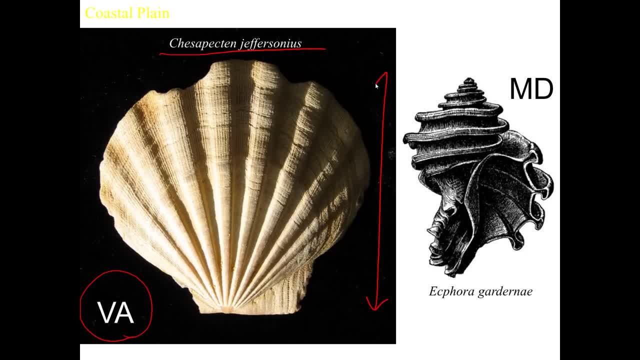 This is a very handsome scallop. It's about 5 or 6 inches from stem to stern. It has historical value because this was the very first fossil that was described in a scientific paper from the New World, Maryland's state fossil is also a mollusk. 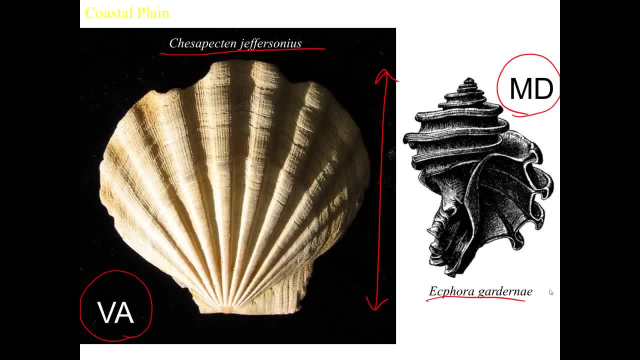 In this case it's a snail Echphora gardneri, a very handsome snail indeed with these four very distinctive ribs that wrap around the snail's structure. Maryland actually only has a few spots where you can find this snail. 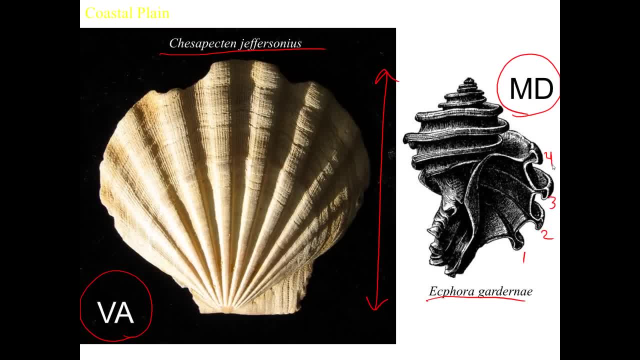 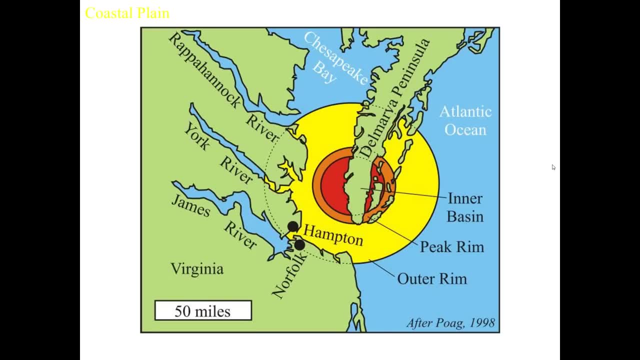 cropping out locally, and Virginia has about 18 spots where you can discover it for yourself. Another thing I'd like you to know about the coastal plain is that it is the hiding place of the United States of America's largest meteorite crater, The Chesapeake Bay impact crater. 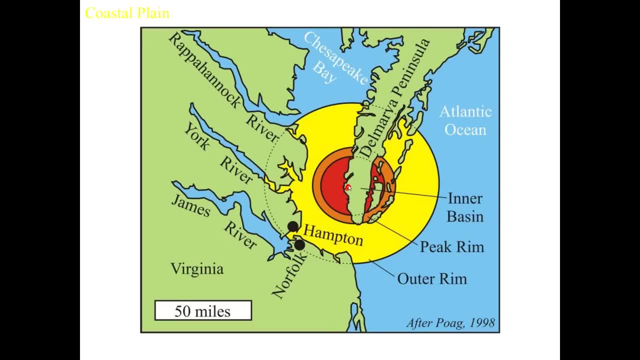 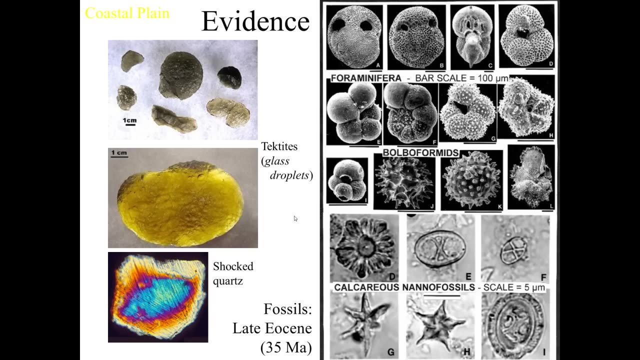 is underneath the Chesapeake Bay, centered on Cape Charles on the Delmarva Peninsula, and it is something like 50 miles in diameter. You can see that it includes both Norfolk and the city of Hampton within its crater range. This was discovered due to the presence of 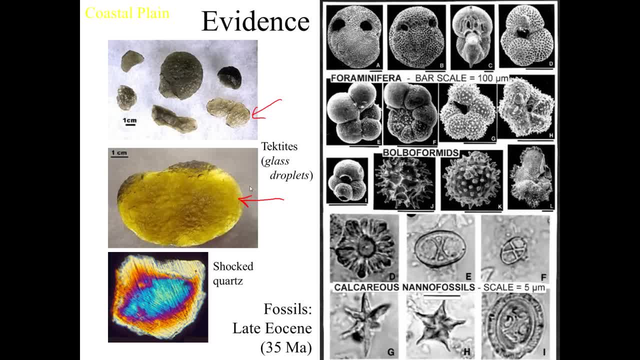 tektites. these are little glass droplets where molten rock was flung into the air and it cooled the glass before it hit the ground, as well as shocked quartz. These were found, actually, originally off the coast of New Jersey, so that's as far away as the stuff landed. 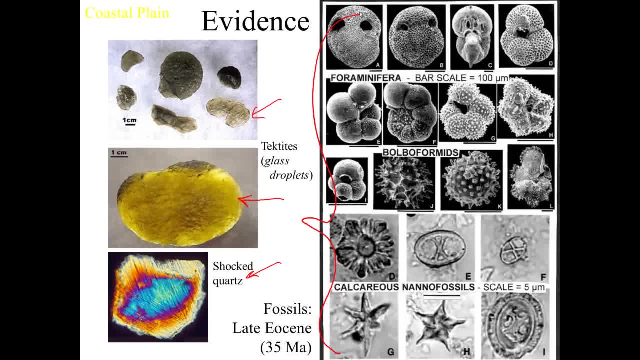 Fossils found in those same sediments allowed geologists to figure out that the impact must have occurred in the late Eocene, around 35 million years ago. This is a search for the crater. Coring, done over on the eastern shore, penetrated an amazing breccia. 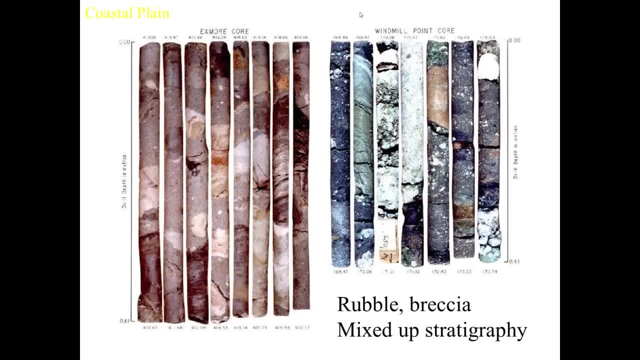 a rubbly rock, that was all sort of mixed up and that breccia shown here in these cores was the signature of the broken up material that filled the crater after the impact. The crater has since been found underneath the Chesapeake Bay. 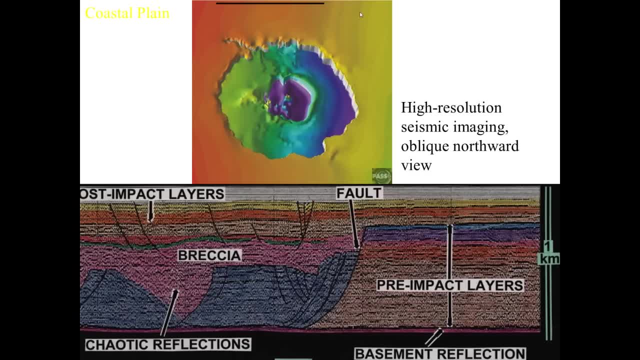 It has been imaged using seismic, where we basically send sound waves down through the layers of sedimentary rock to find its structure. You can see this overall depressed shape with a central little peak that has rebounded, kind of shaped like a sombrero. 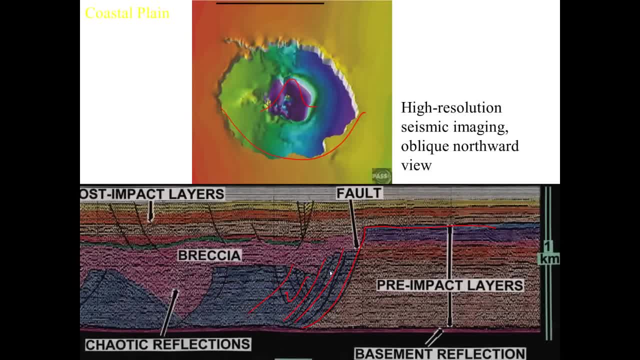 You've got pre-impact layers that then had faults, where materials collapsed into the crater hole, and then all that breccia material fell back into the hole as well. After the impact, things returned to normal calm, passive margin sedimentation. 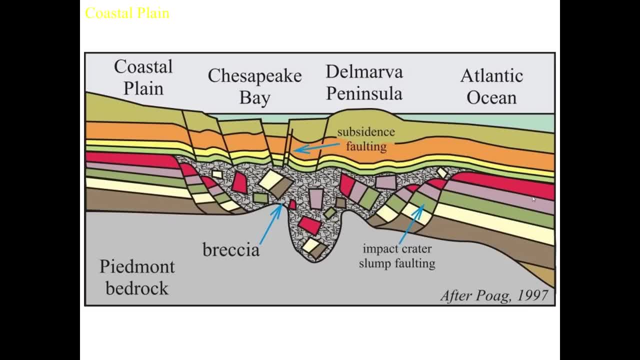 and you've got post-impact layers on top. So the overall cross section through the Chesapeake Bay region shows the Piedmont bedrock down below the pre-impact layers. on top of that, the impact itself with that crater and then the rubble filling the crater. 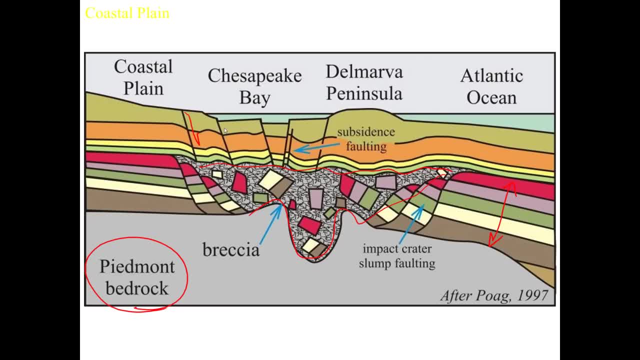 the breccia And then the post-impact layers have seen a little bit of faulting as the breccia has compacted over time. That faulting has created a low-lying area, and that's why the Chesapeake Bay is where the Chesapeake Bay is.